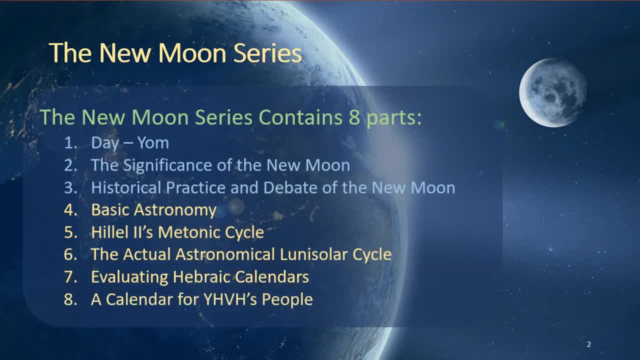 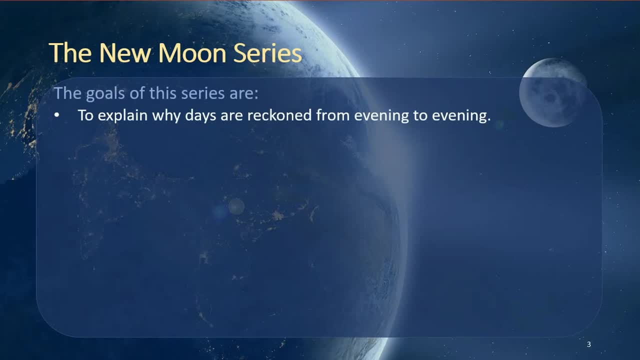 Evaluating Hebraic Calendars And, finally, a calendar for Yehovah's people. The goals of this series are to explain why days are reckoned from evening to evening, To teach the significance of the New Moon and its impact on reckoning the first day of the month. 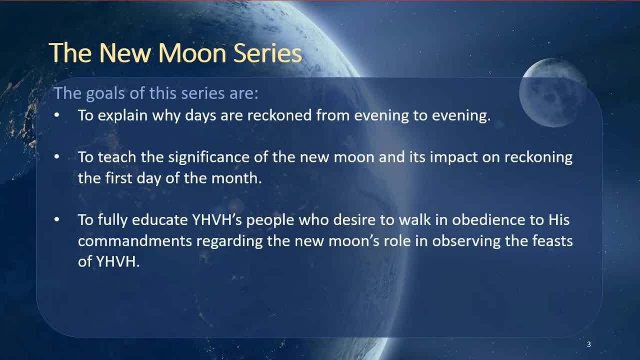 Also to fully educate Yehovah's people who desire to walk in obedience to his commandments. regarding the New Moon's role in observing the Feast of Yehovah, Also to introduce and address the debate over Conjunction vs New Crescent Moon. 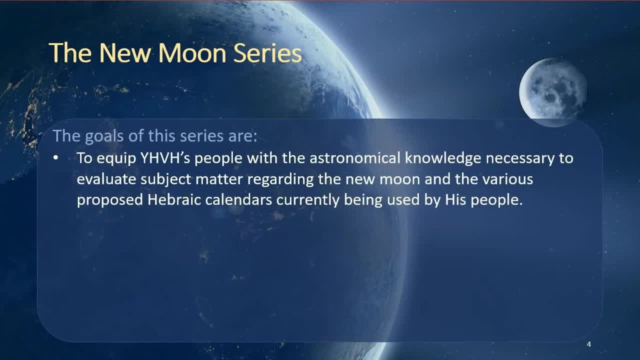 To equip Yehovah's people with the astronomical knowledge necessary to evaluate subject matter regarding the New Moon and the various proposed Hebraic calendars currently being used by his people. Also, to propose a Hebraic calendar that Yehovah's people worldwide can follow without reliance on other assemblies. 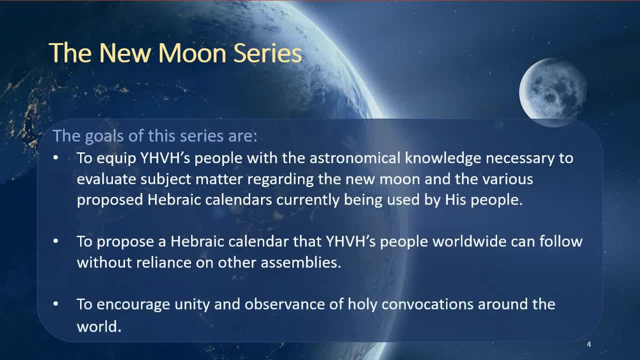 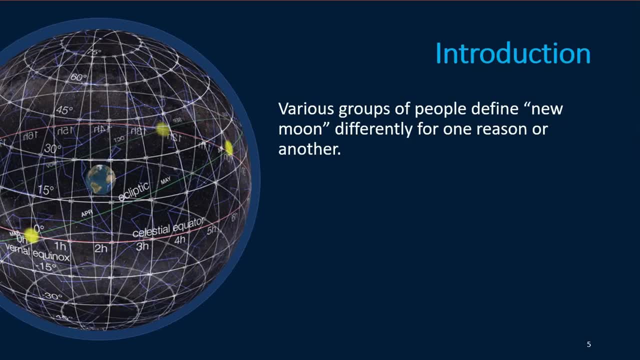 And finally, to encourage unity and observance of holy convocations around the world. Various groups of people define New Moon differently, for one reason or another, And we talked about that previously in another presentation. Astronomers define the New Moon as Conjunction. 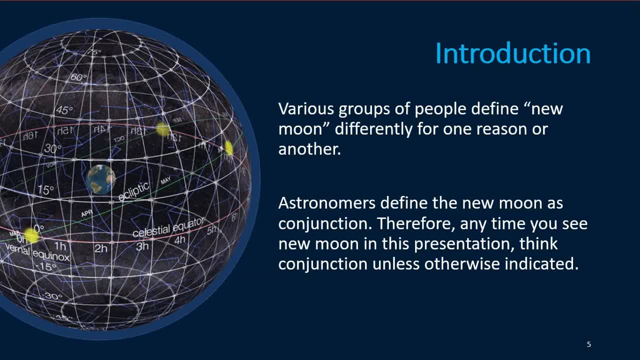 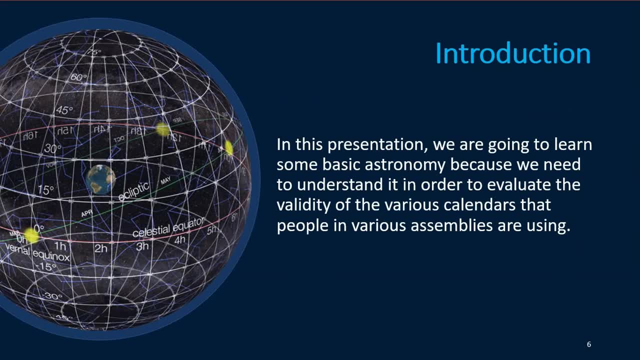 Therefore, anytime you see the New Moon in this presentation, think of it as Conjunction, And you can find out more about the New Moon in this presentation. think conjunction. unless otherwise indicated In this presentation we're going to learn some basic astronomy because we need to understand it in order to evaluate the validity of the 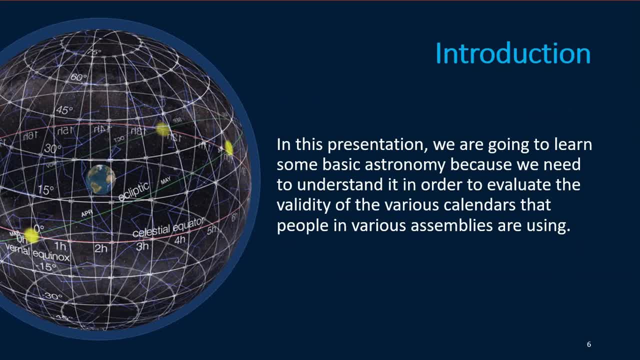 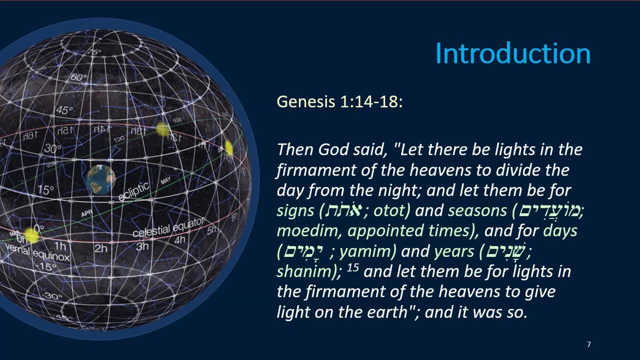 various calendars that people in various assemblies are using. Genesis 1,, 14 through 18 says. Then God said: Let there be lights in the firmament of the heavens to divide the day from the night, and let them be for signs and seasons and for days and years, and let 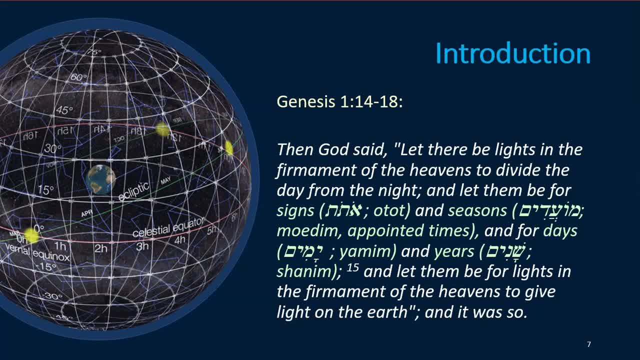 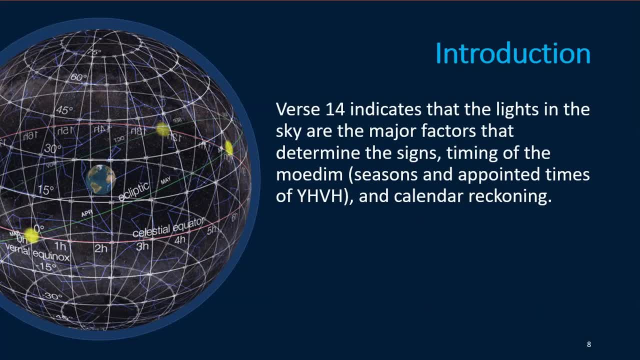 them be for lights in the firmament of the heavens to give light on the earth, And it was so. Verse 14 indicates that the lights in the sky are the major factors that determine the signs. timing of the Moedim, which are the seasons and appointed times of Yehovah. 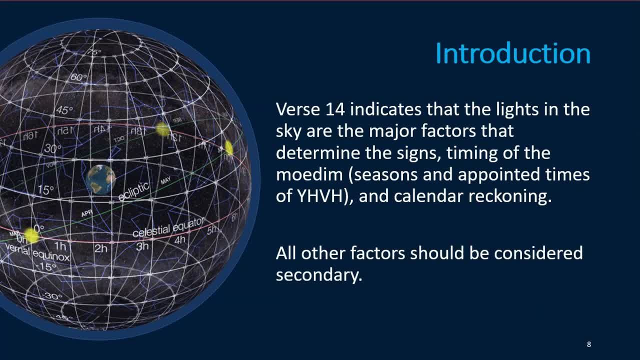 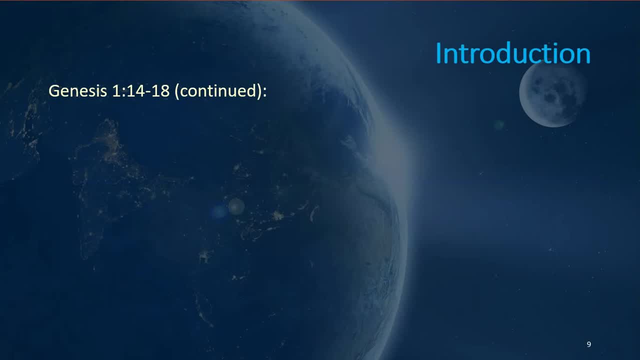 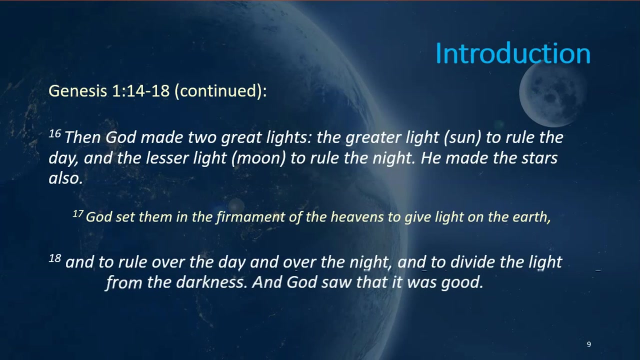 and calendar reckoning. All other factors should be considered separately. Now let's continue with Genesis 1,, 14 through 18.. And God saw that it was good. Notice how the chiasm of verses 16 through 18 points to the 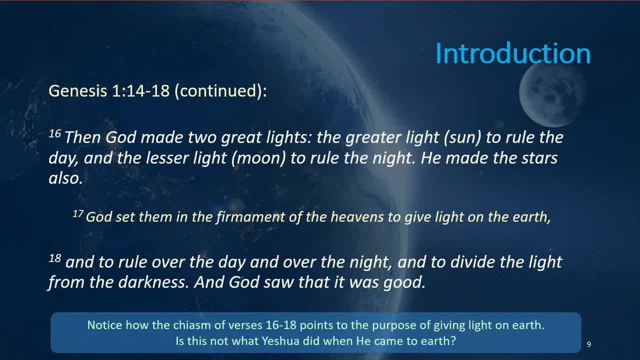 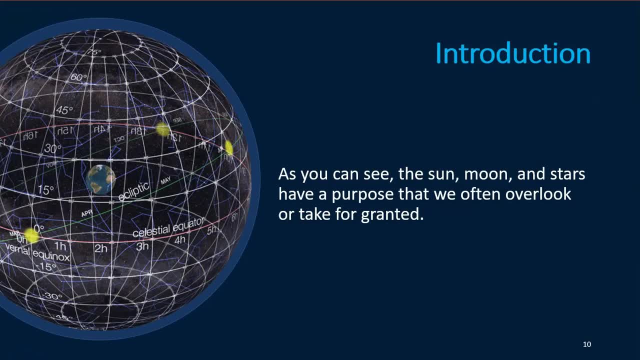 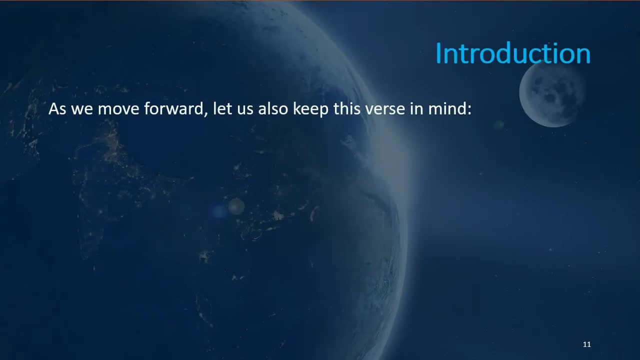 purpose of giving light on earth. Is this not what Yeshua did when he came to the earth? As you can see, the sun, moon and stars have a purpose that we often overlook or take for granted. As we move forward, let's also keep this verse in mind. 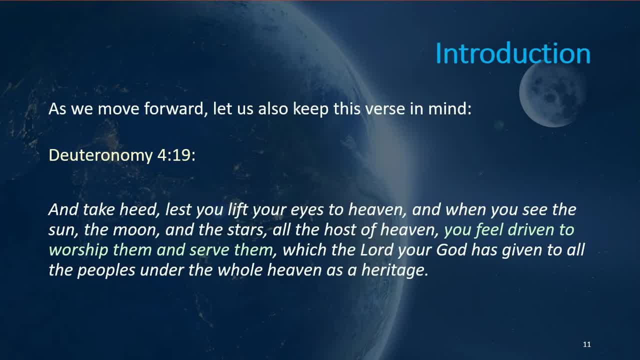 Deuteronomy 4, 19.. And take heed lest you lift your eyes to heaven and when you see the sun, the moon and the stars, all the hosts of heaven, you feel driven to worship them and serve them. 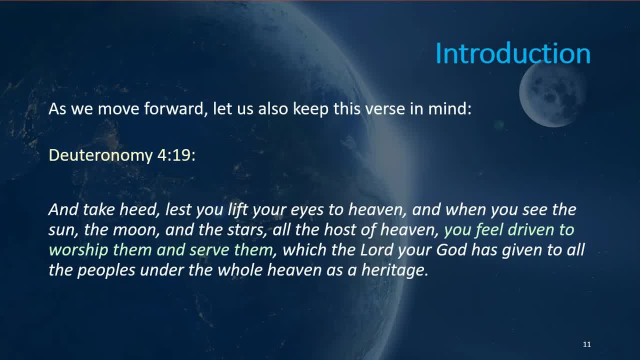 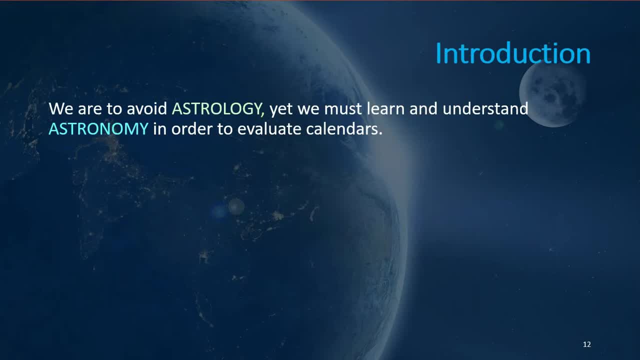 which the Lord, your God, has given to all the peoples under the whole heaven as a heritage. We're to avoid astrology, yet we must learn and understand astronomy in order to evaluate calendars. The key difference is that astrology involves worship of the celestial bodies, not of the celestial bodies, So we must learn and understand astronomy. 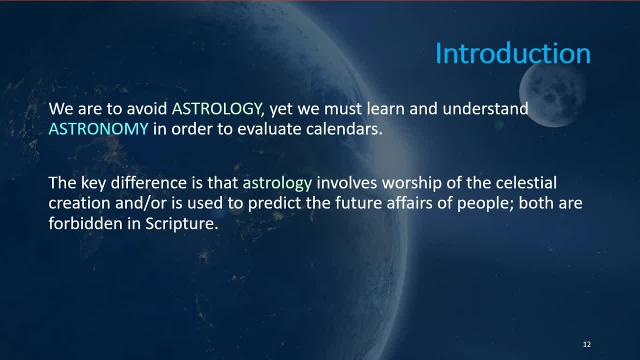 and the celestial creation and or is used to predict the future affairs of people, and both are forbidden in scripture. Astronomy, on the other hand, is a study of the celestial bodies and how they operate together, and that's what we want to focus on. 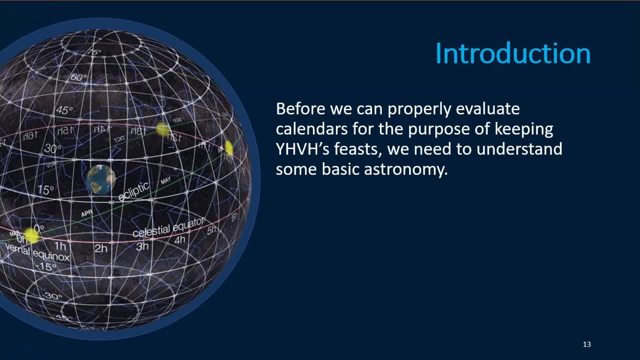 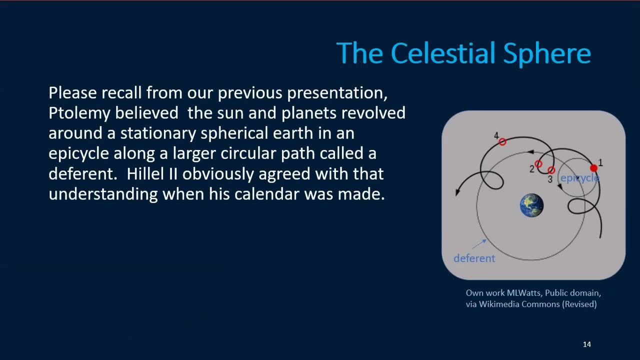 Before we can properly evaluate calendars for the purpose of keeping Yehovah's feasts, we need to understand some basic astronomy. As I've already said, this presentation will lay the foundation to do just that. Please recall from our previous presentation: Ptolemy believed the sun and planets revolved. 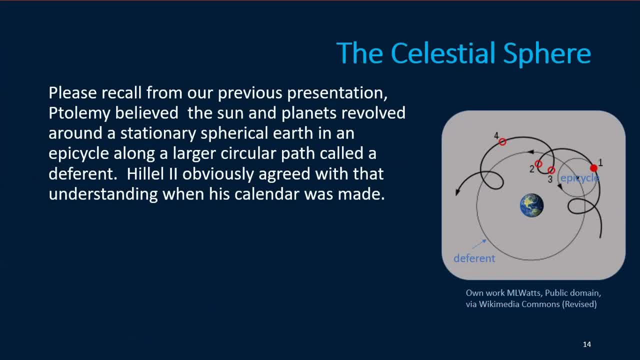 around a stationary spherical earth in an epicycle along a larger circular path called a deferent. Hillel too, obviously agreed with that understanding when his calendar was made. Also, remember, it was widely accepted by the 5th century BCE that the sun and planets revolved around a stationary spherical earth in an epicycle along a larger circular path called a deferent. 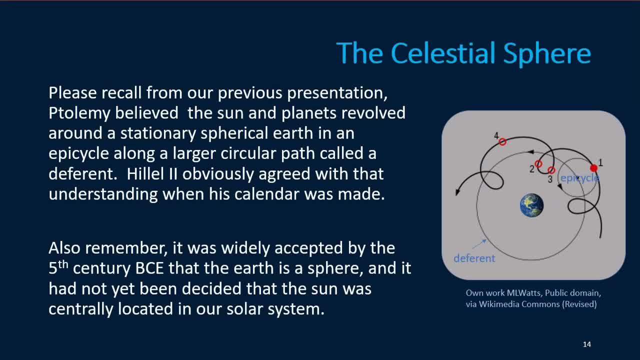 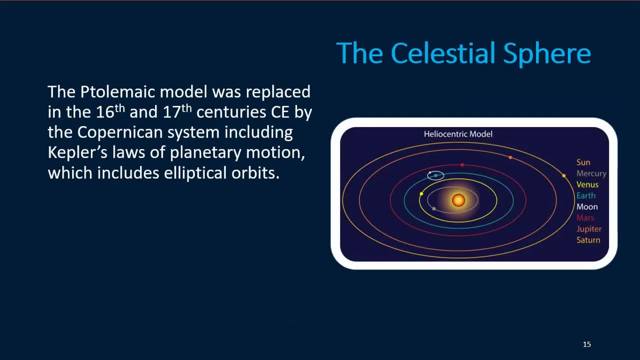 That the earth is a sphere and it had not yet been decided that the sun was centrally located in our solar system. The Ptolemaic model was replaced in the 16th and 17th centuries Common Era by the Copernican system, including Kepler's laws of planetary motion, which includes elliptical orbits. 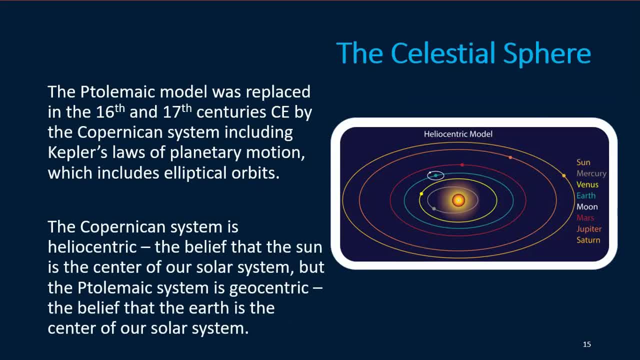 The Copernican system is heliocentric- the belief that the sun is the center of our solar system- but the Ptolemaic system is geocentric- the belief that the earth is the center of our solar system. Both of these systems recognize a spherical earth. 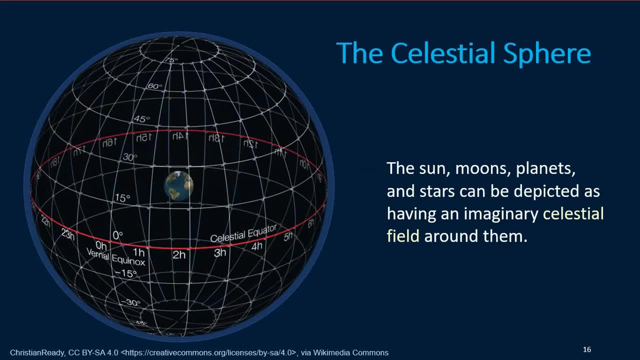 The sun, moons, planets and stars can be depicted as having an imaginary celestial field around them. This makes it easier to locate things in space using a coordinate system similar to that of a globe's latitude and longitude coordinate system. The planet's position is created by a nuclear system. 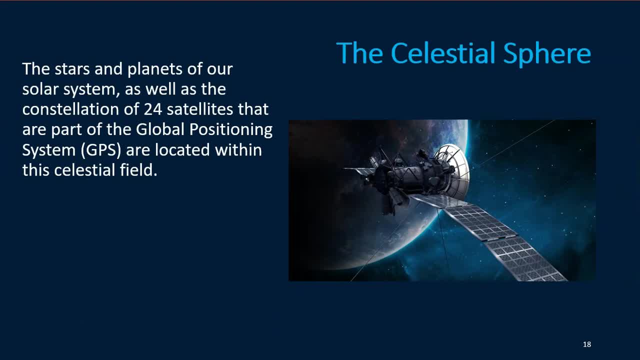 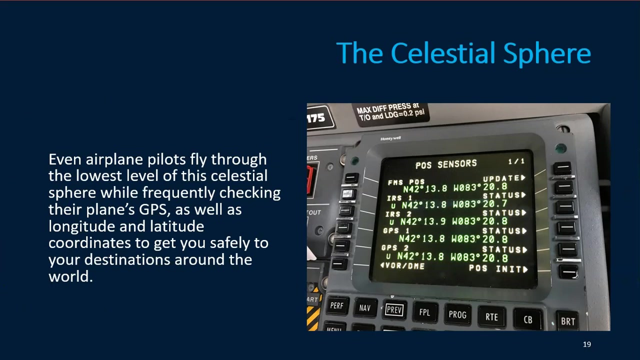 and also by a quantum pair, both of which are possible by entering a certain of the common surface surface. And here it is, aApprov바, a very, very test: 수가ν CrutIncE crawling akan, sailing� 79 degrees up the rock's area. The planets and planets in the solar system, as well as the constellation of 24 satellites that are part of the global positioning system, are located within this celestial field. These satellites can report their positions in the celesttial field and can be maneuvered into new positions by the control segment of the global position system. You're welcome to exploreah AskScicom if. 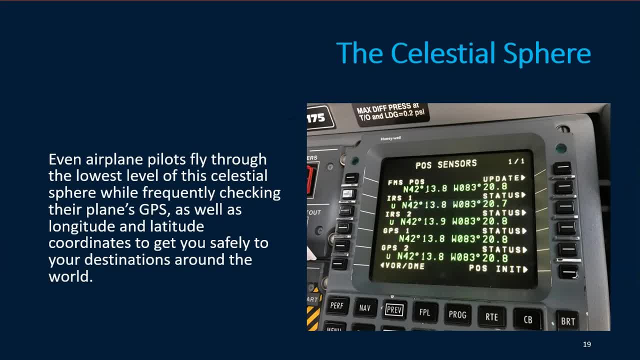 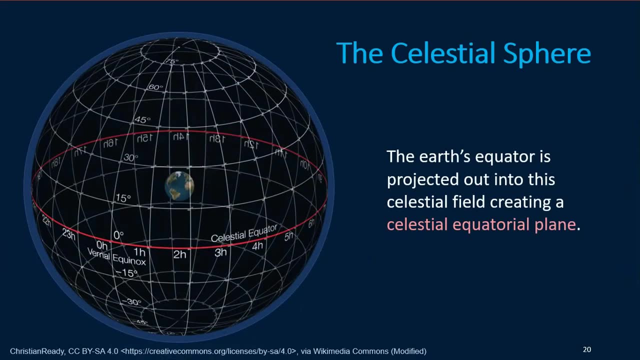 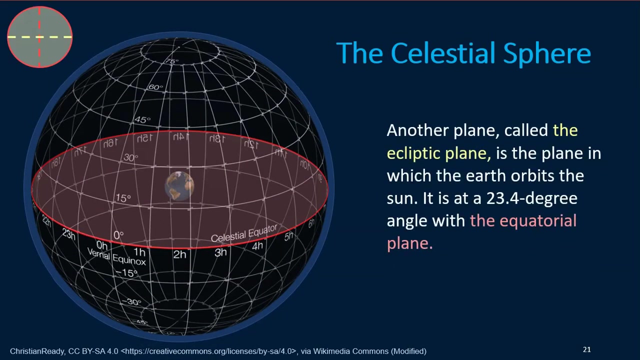 this celestial sphere while frequently checking their plane's GPS as well as longitude and latitude coordinates to get you safely to your destinations around the world. The Earth's equator is projected out into this celestial field, creating a celestial equatorial plane. Another plane, called the ecliptic plane, is the plane in which the Earth orbits. the 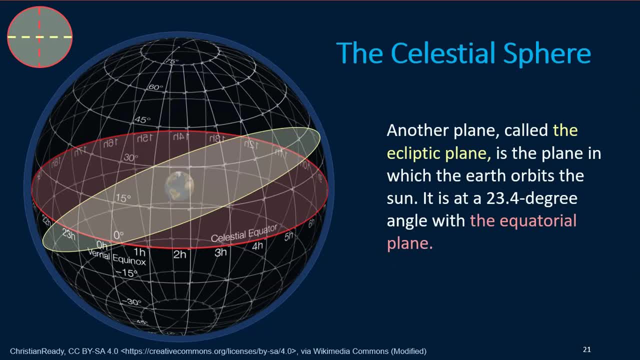 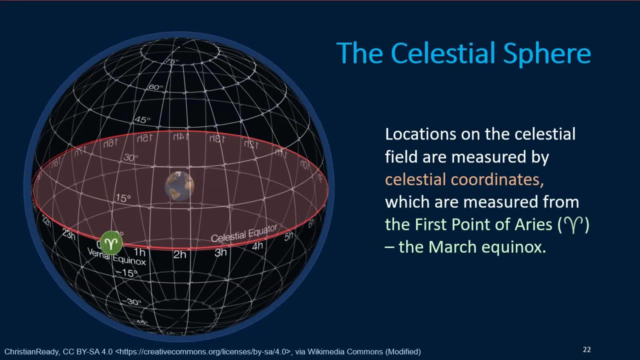 Sun. It is at a 23.4 degree angle with the equatorial plane. Locations on the celestial field are measured by celestial coordinates, which are measured from what's called the first point of Aries. This is also known as the March Equinox. 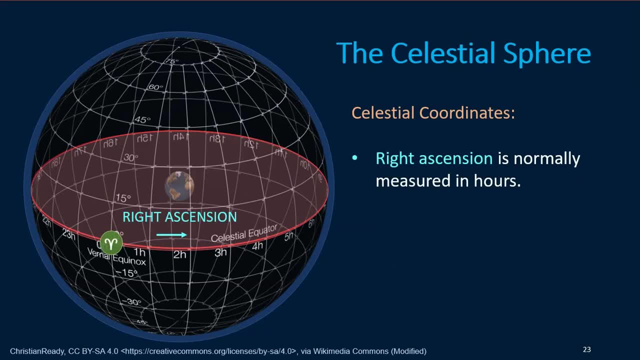 The celestial coordinates are composed of two measurements. The first one is the right ascension, and it's normally measured in hours as it moves around the celestial field. There are a total of 24 hours of right ascension. Declination is measured in degrees plus 90 degrees above the equatorial plane and negative. 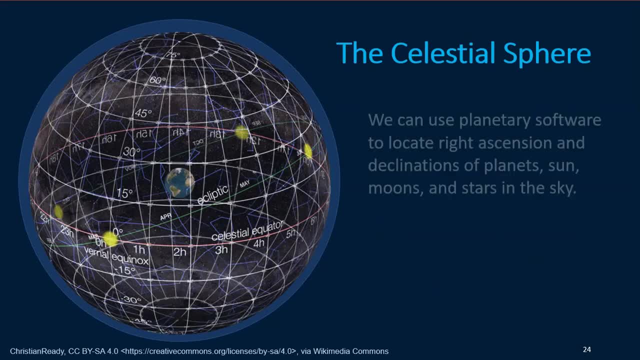 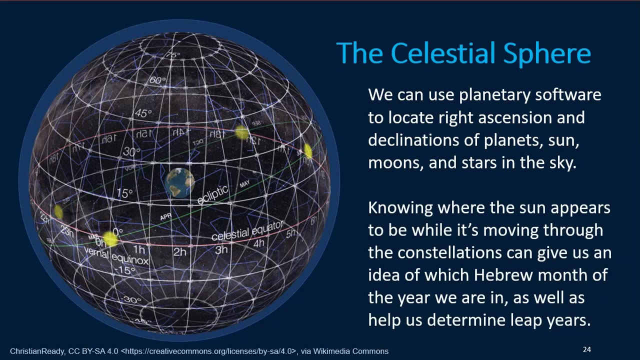 90 degrees below the equatorial plane. We can use planar planetary software to locate right ascension and declinations of planets, sun moons and stars in the sky, Knowing where the Sun appears to be while it's moving through the constellations can. 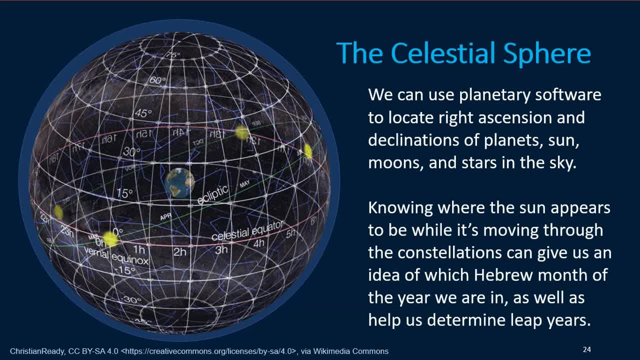 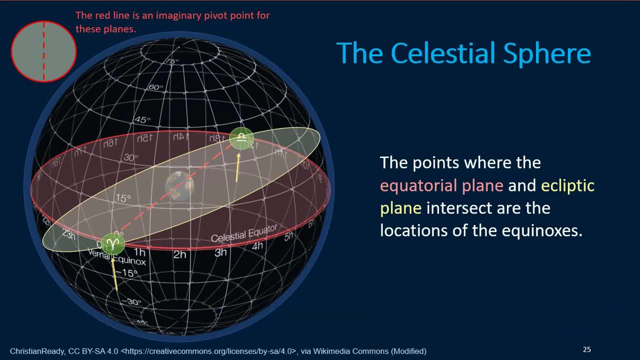 give us an idea of which Hebrew month of the year we're in, as well as help us determine leap years. The points where the equatorial plane and the ecliptic plane intersect are the locations of the equinoxes. This red line is an imaginary pivot point for these planes. 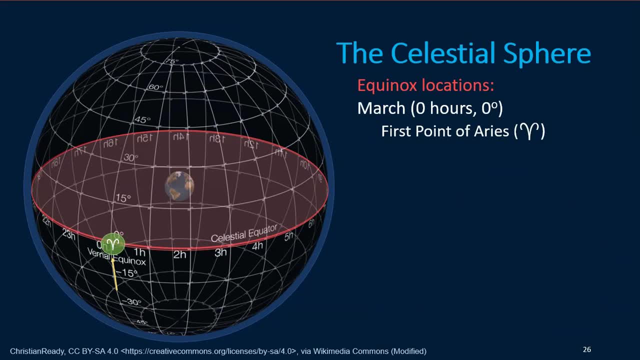 Let's take a look at the equinox and solstices locations on our celestial field. We'll begin with the March Equinox. This is also known, by the way, as the Vernal Equinox or the Spring Equinox, And I keep referring to this more as the March Equinox because I'm also aware that what's 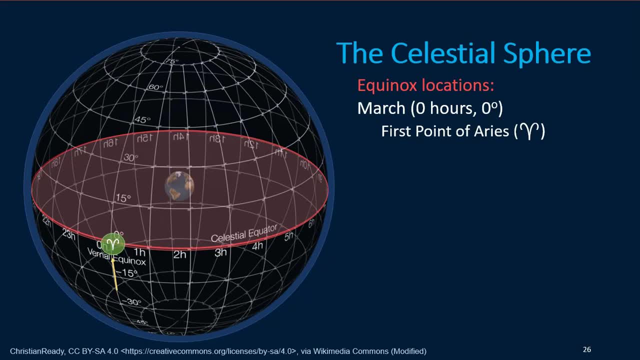 going on in the Southern Hemisphere, Seasons wise, is different from that of the opposite hemisphere. Our first location, and probably the most important, is the March Equinox, which is also known as the first point of Aries. It's located at zero hours of right ascension and zero degrees of declination. 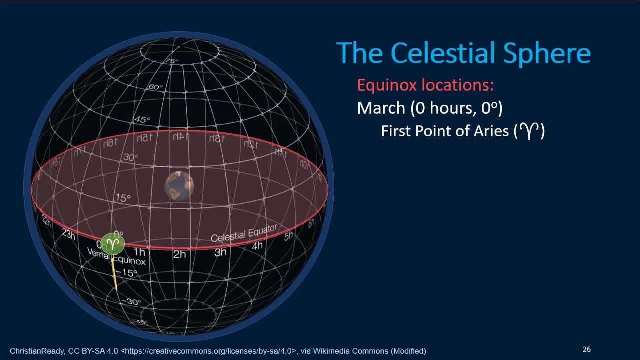 And as we're looking at this sphere, I am trying to explain a three dimensional idea. It's in a one dimensional picture, So I'm going to do my best to kind of explain this as we're looking at it, so you can kind of conceptualize this perhaps a little bit better in your mind. 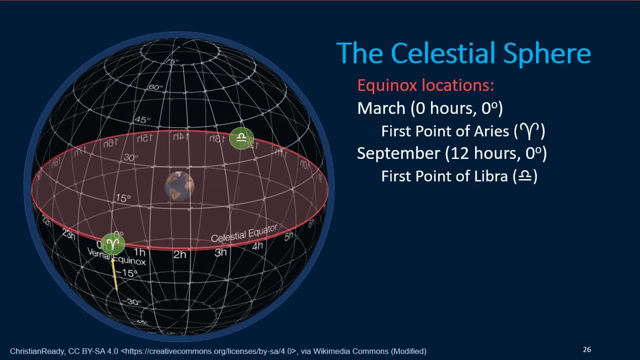 The September Equinox is located at 12 hours of right ascension and zero degrees of declination. It's also known as the first point of Libra. It's located in the back of our celestial field. It is- It's the first point of the first point of Aries. 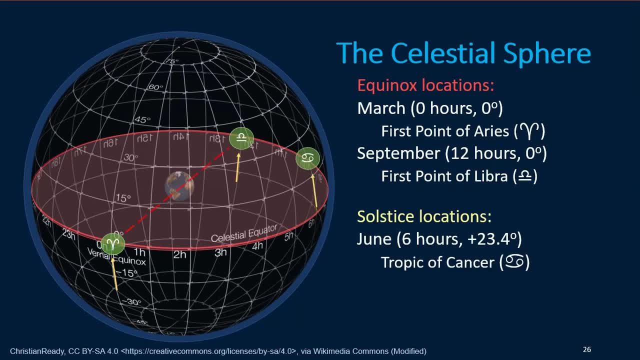 Now we'll look at the solstice locations. The first one is going to be the June solstice. It's located at six hours of right ascension, but it's located at positive 23.4 degrees of declination. So when we're looking at it we're going to come over here to the six hour mark, which 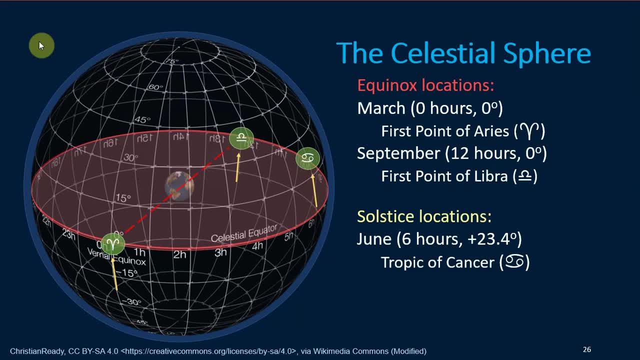 is really between the Equinox location. I'm going to go through the locations as far as right ascension goes- although it does not really appear that way on this picture, It is. And then it's elevated higher than the equatorial plane. 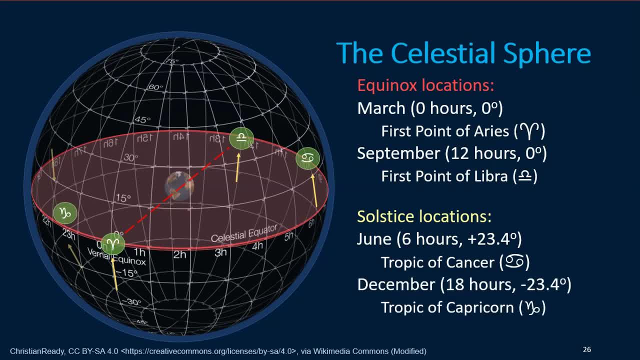 So it would go up this way. Then the December solstice is located at 18 hours of right ascension, And in this picture it does look like it's more forward, But really it's back a bit. so if you look at the arrows you kind of imagine that a little bit further back. 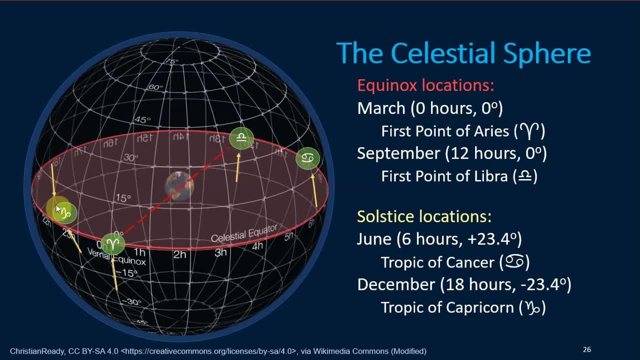 and so we have opposite lines going that way, and then when I actually put the plane in there, you can kind of see, maybe a little bit, how it is raised up a bit, and I don't want you to have the idea that it's more oval necessarily than the other, but perhaps, if you 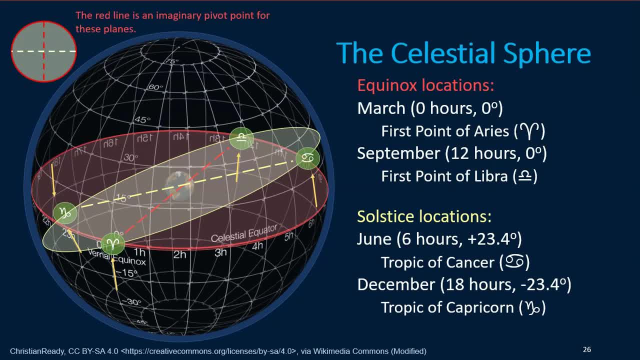 look at it this way: on this little circle in the upper left you can kind of see how they overlap each other in a way, and we are showing this celestial field kind of at a different angle, with the beginning kind of starting a little bit more toward the left than the right. 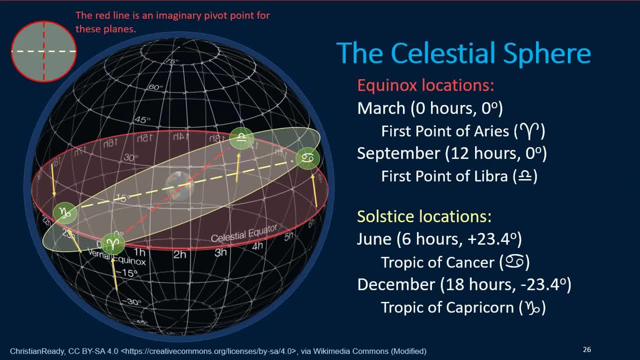 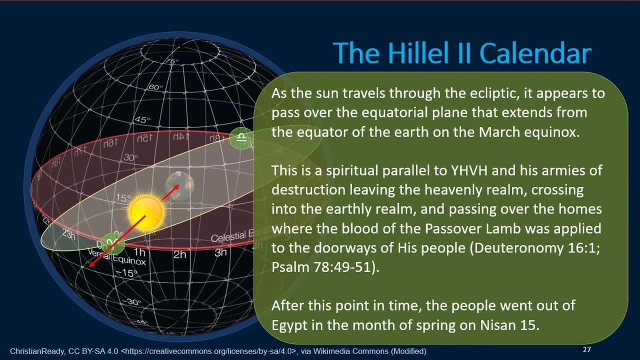 and not really in the center. As the sun travels through the ecliptic, it appears to pass over the equatorial plane. that extends to the south. It extends from the equator of the earth on the march equinox and this, I think, is a spiritual 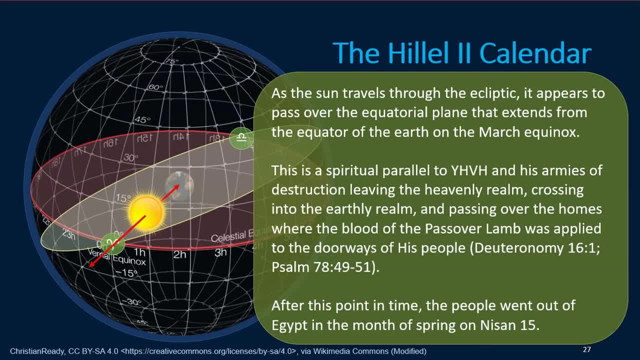 parallel to Yehovah and his armies of destruction, leaving the heavenly realm, crossing into the earthly realm and passing over the homes where the blood of the Passover lamb was applied to the doorways of his people. and as we think about that, we also need to compare and contrast what's. 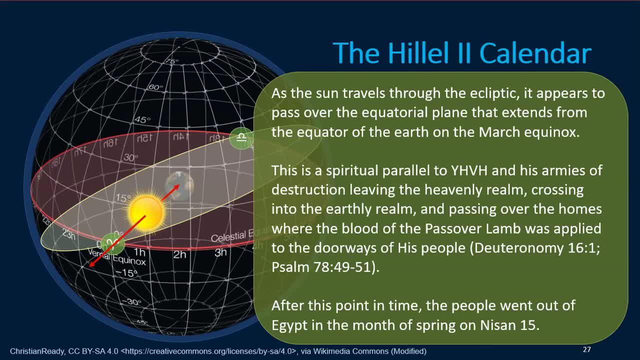 found in Deuteronomy 16: 1 and Psalm 78 49.. Because it was not really Yehovah who was going in and destroying all these people, but he actually had an army with him that was doing the destruction. and after this point in: 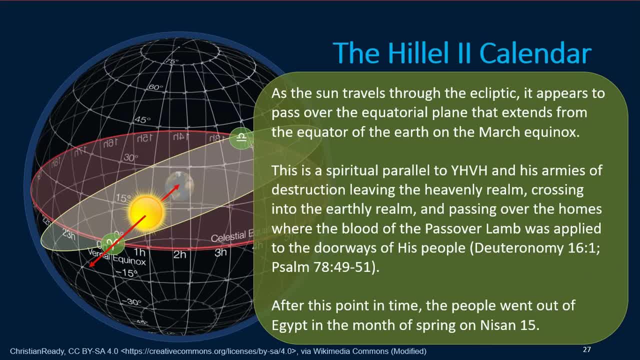 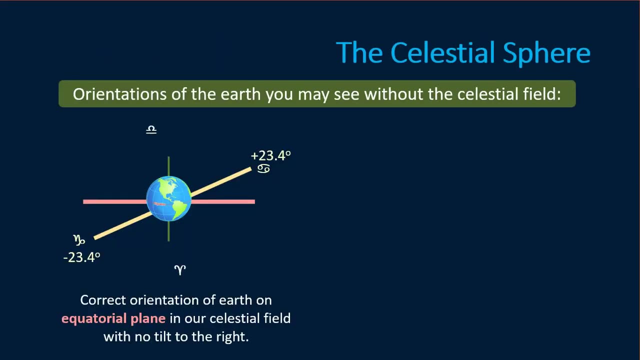 time. the people went out of Egypt in the month of spring, on Nisan 15th, and this concept becomes a very important point when we're considering when the beginning of spring is, or the beginning of Aviv. Okay, there's a couple of orientations of the earth that you may see without the celestial field. 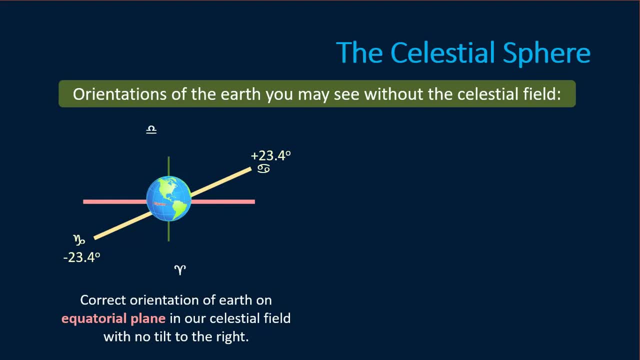 The first one looks like this one on the left. This is the correct orientation of the earth on the equatorial plane in our celestial field, with no tilt to the right, and basically what we've done is removed that celestial field and then a lot of drawings that you'll see online. you'll see: 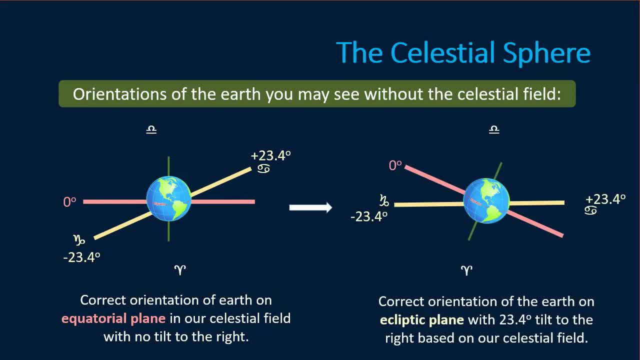 something that looks like this, where the ecliptic plane is made to appear in that horizontal position. So, basically, what you have is the correct orientation of the earth on the ecliptic plane, with a 23.4 degree tilt to the right, based on our 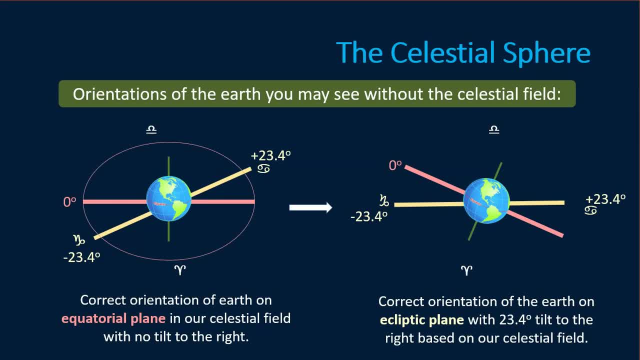 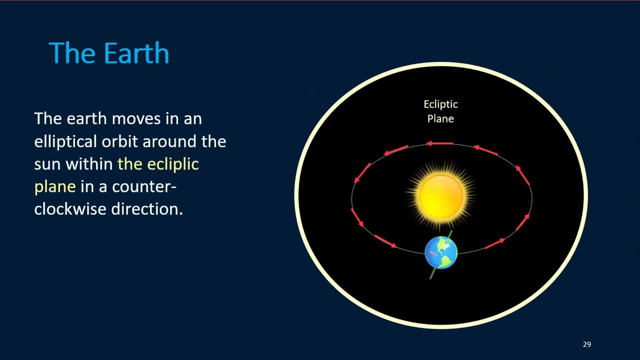 celestial field. So it would look like that. and then, if we were to add our planes, it could look even like this: The earth moves in an elliptical orbit around the sun, with the ecliptic plane In a counterclockwise direction. a 23.4 degree tilt of the earth is always maintained as it's. 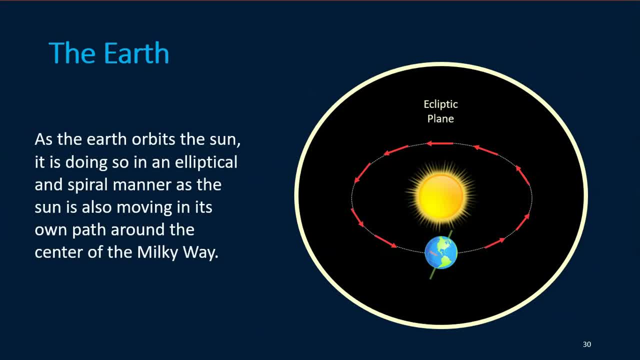 orbiting the sun. As the earth orbits the sun, it's doing so in an elliptical and spiral manner, as the sun is also moving in its own path around the center of the milky way. As the earth orbits the sun, the earth is spinning eastward on its imaginary tilted axis, and one revolution of the 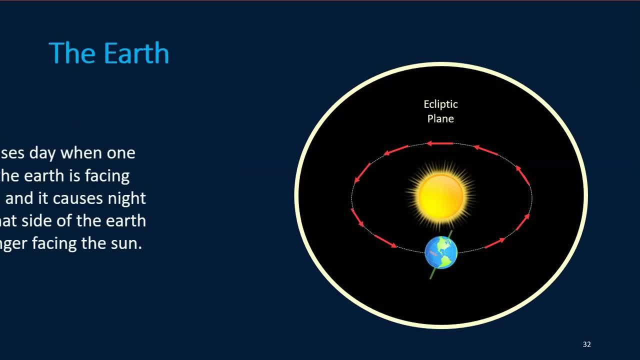 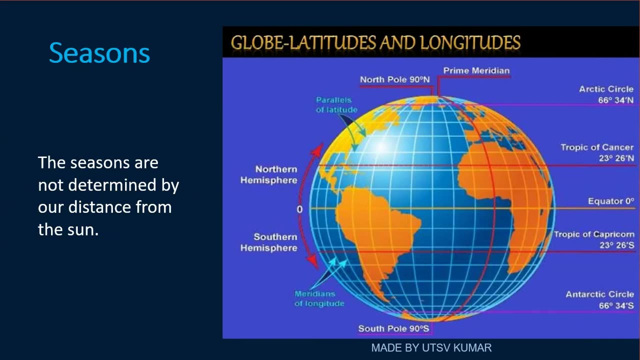 earth on its imaginary tilted axis, is spinning eastward on its imaginary tilted axis. This causes day when one side of the earth is facing the sun, and it causes night when that side of the earth is no longer facing the sun. The seasons are not determined by our distance from the Sun. They're determined by the tilt. 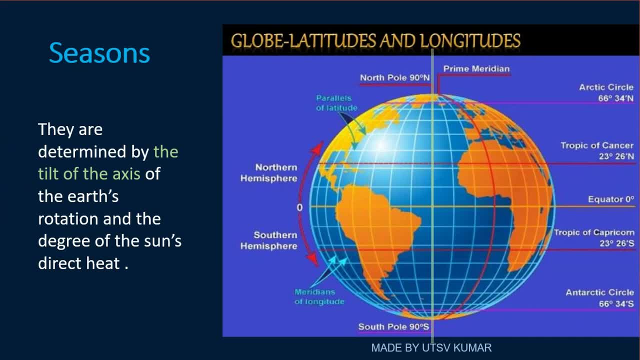 of the axis of the earth's rotation and the degree of the sun's direct heat. During the equinoxes, the sun is directly facing the equator and the sun is directly facing the equator. During the equinoxes, the sun is directly facing the equator and the sun is directly facing the equator. 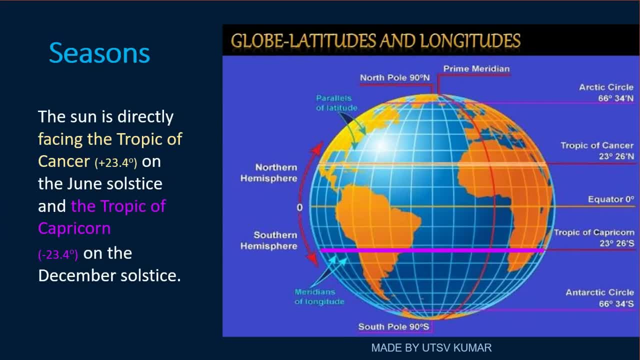 The sun is directly facing the Tropic of Cancer, or positive 23.4 degrees on the June solstice, and the Tropic of Capricorn, which is the negative 23.4 degrees on the December solstice. The sun is directly facing the Tropic of Cancer, or positive 23.4 degrees on the June solstice, and the Tropic of Capricorn, which is the negative 23.4 degrees on the December solstice. 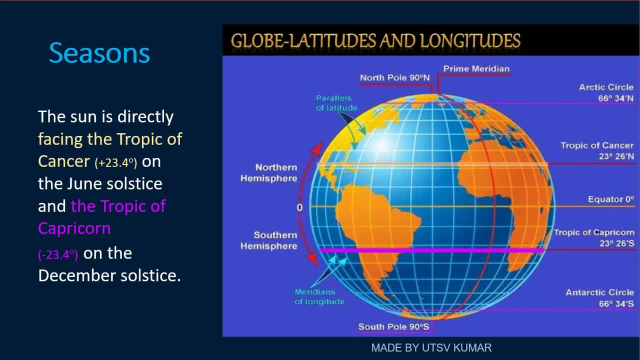 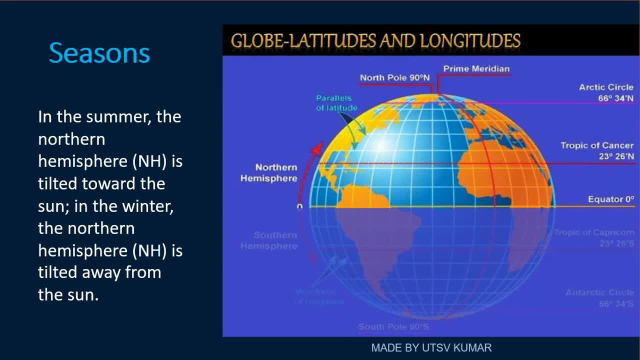 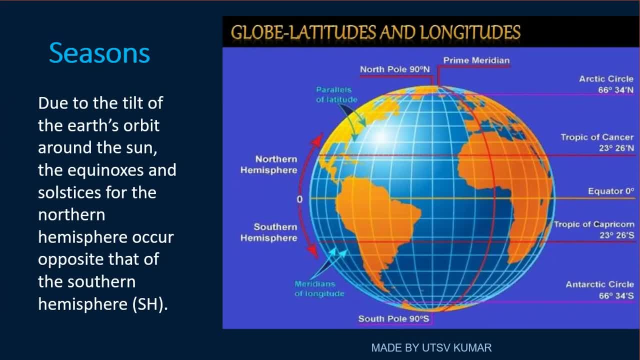 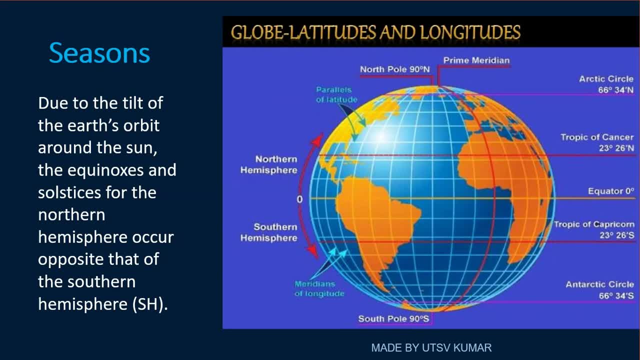 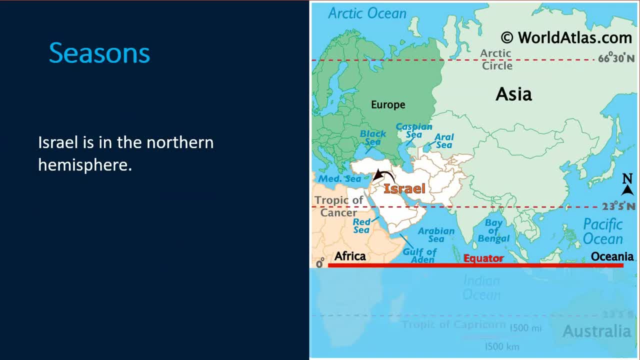 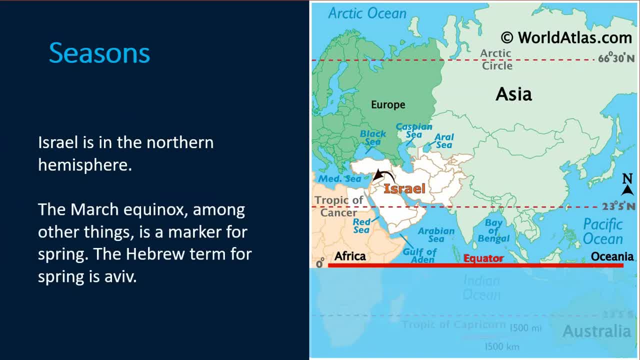 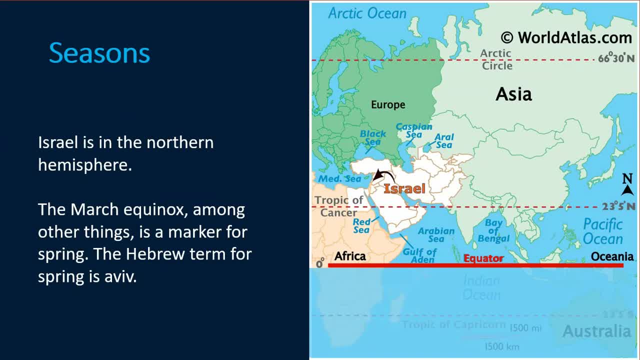 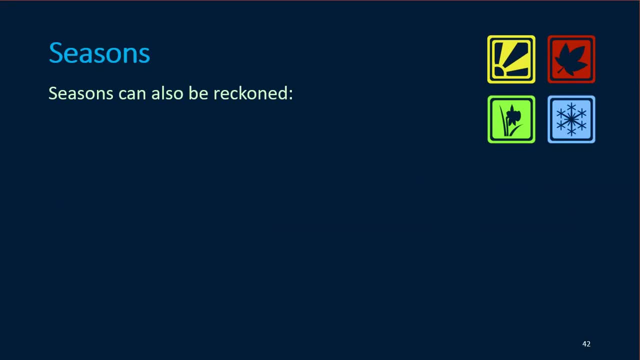 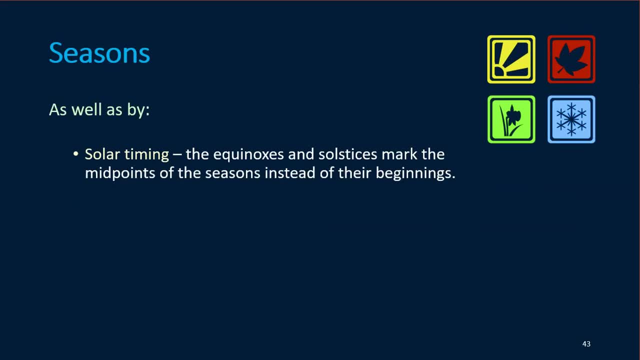 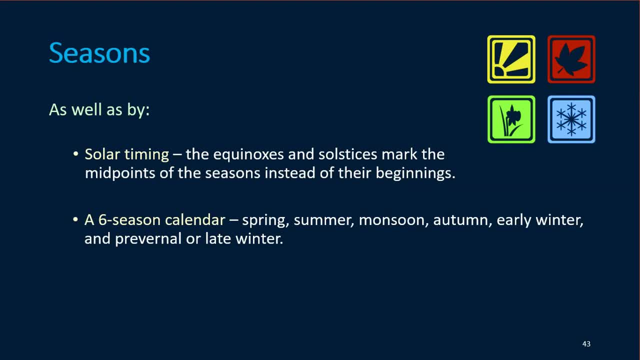 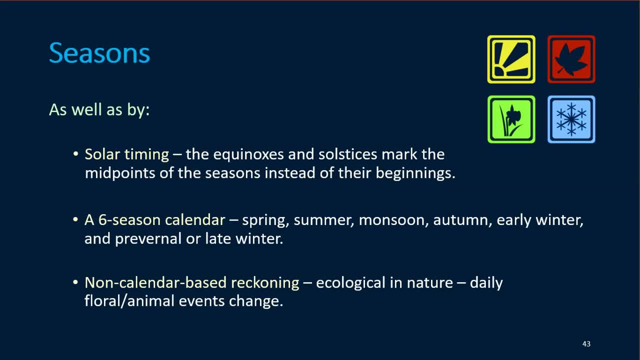 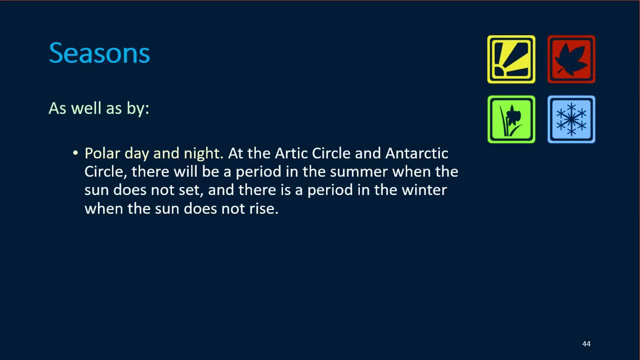 The sun is directly facing the Tropic of Cancer, or positive 23.4 degrees on the June solstice. The sun is directly facing the Tropic of Cancer, or positive 23.4 degrees on the June solstice. There will be a period in the summer when the sun does not set and there is a period in the winter when the sun does not rise. 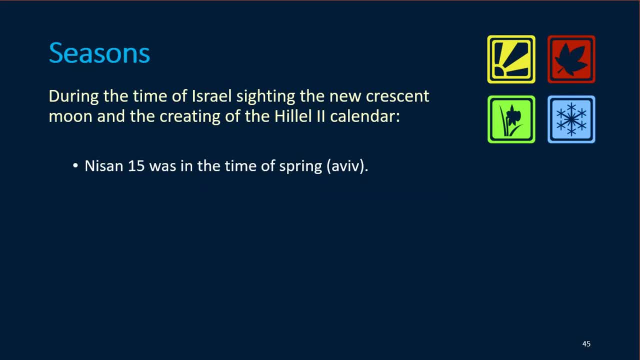 During the time of Israel, sighting the new crescent moon and the creating of the Hillel 2 calendar. Nisan 15 was in the time of spring. If the equinox fell before what would be the 16th of Nisan, the year was a regular year, and this regular year had 12 months. 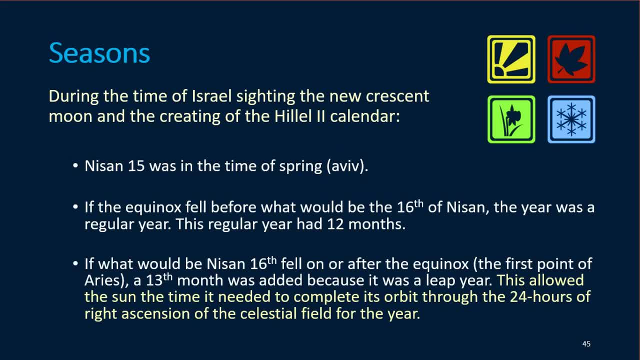 If what would be Nisan's 16th fell on or after the equinox, the first point of Aries, a 13th month was added because it was a leap year. This allowed the sun the time it needed to complete its orbit through the 24 hours of right ascension of the celestial field for the year. 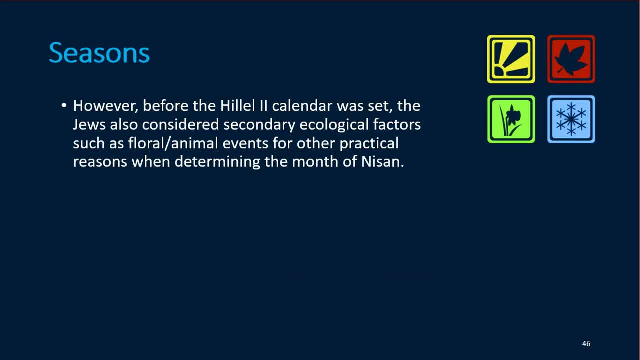 However, before the Hillel 2 calendar was set, the Jews also considered secondary ecological factors such as floodgates. In addition, the leap years of the Hillel 2 calendar are not occurring according to the equinox rule, as they should. 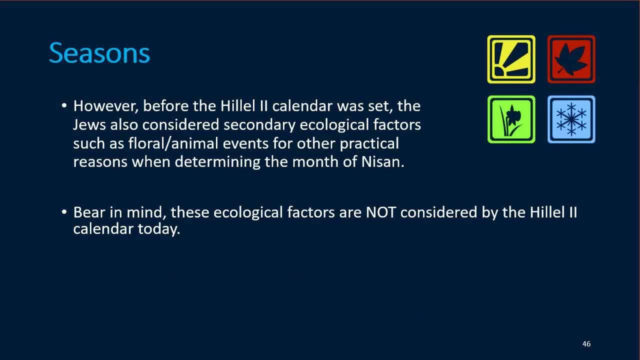 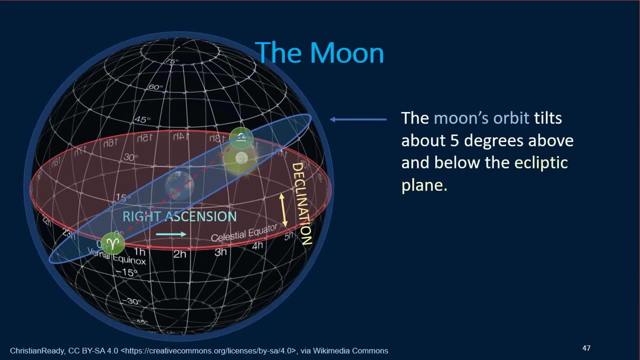 Bear in mind, these ecological factors are not considered by the Hillel 2 calendar today. In addition, the leap years of the Hillel 2 calendar are not occurring according to the equinox rule, as they should. Now let's talk about the moon. 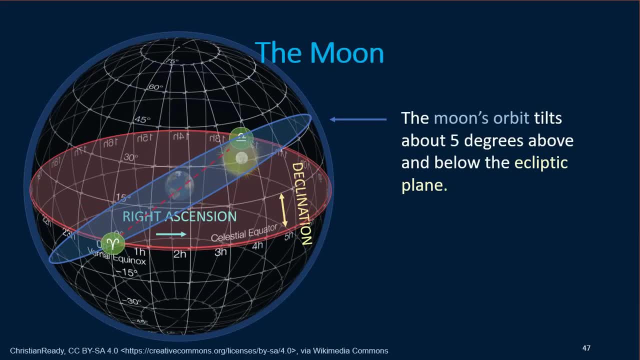 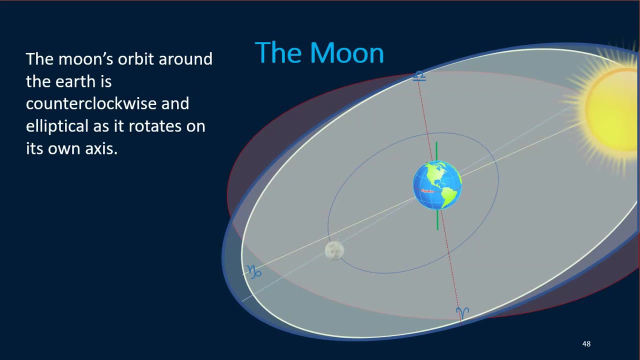 The moon's orbit tilts about 5 degrees above and below the ecliptic plane. This affects how we see the moon in its different phases. The moon's orbit around the earth is counterclockwise and elliptical as it rotates on its own axis. 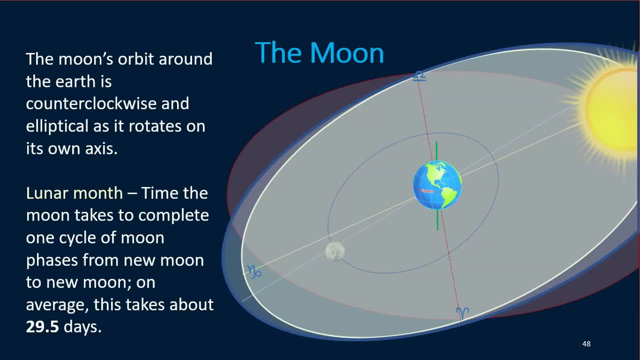 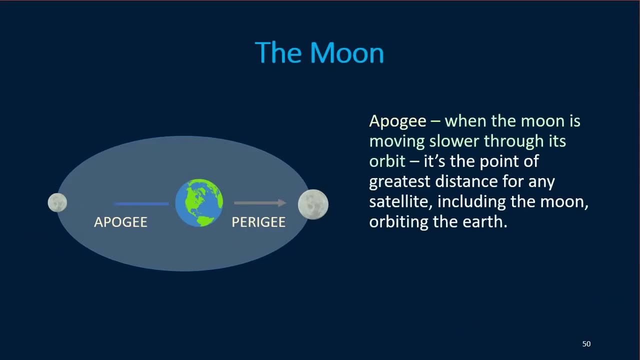 A lunar month is the time the moon takes to complete one cycle of the moon phases, from one new moon to the new moon. On average, this takes about 29.5 days. Apogee is when the moon is rotating, moving slower through its orbit. It's the point of greatest distance for any 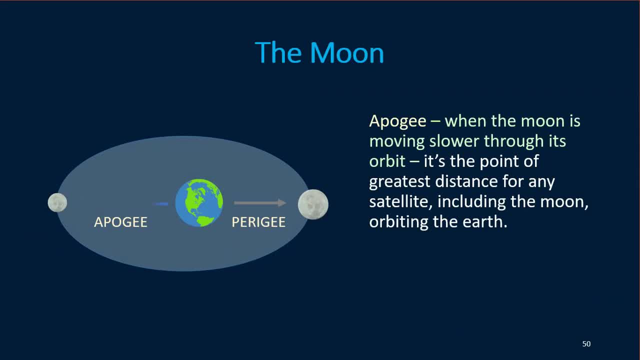 satellite, including the Moon, orbiting the Earth. This is when the micro moon is seen from the Earth. Perigee is when the Moon is moving faster through its orbit. It is the point of least distance for any satellite, including the Moon. 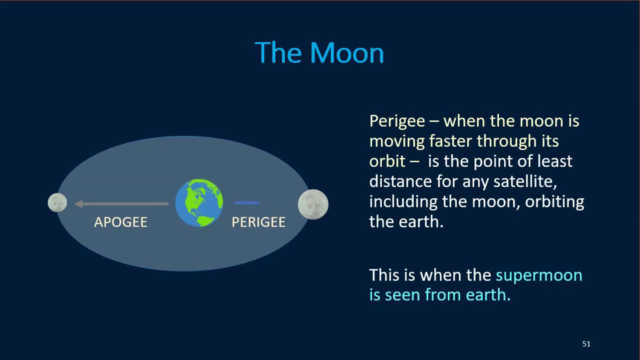 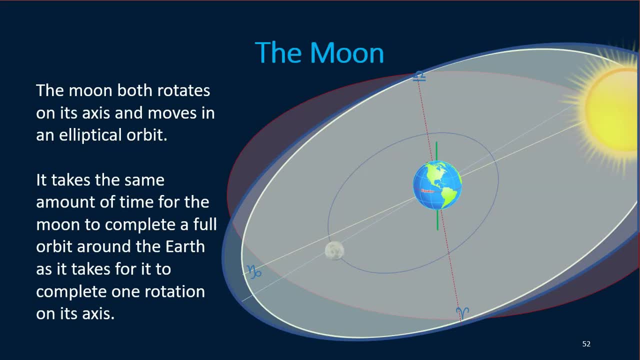 orbiting the Earth. This is when the supermoon is seen from the Earth. The The Moon both rotates on its axis and moves in an elliptical orbit. It takes the same amount of time for the Moon to complete a full orbit around the Earth. 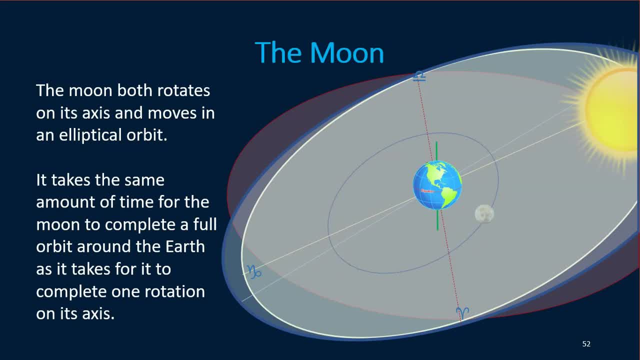 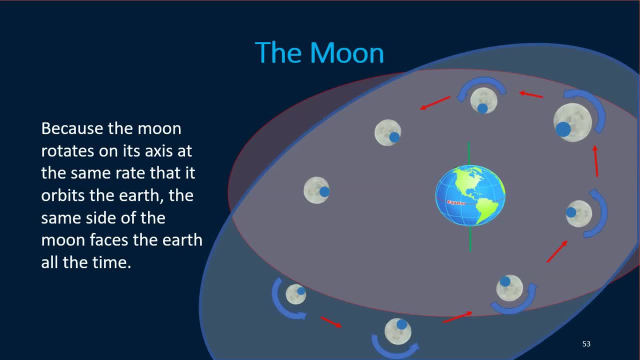 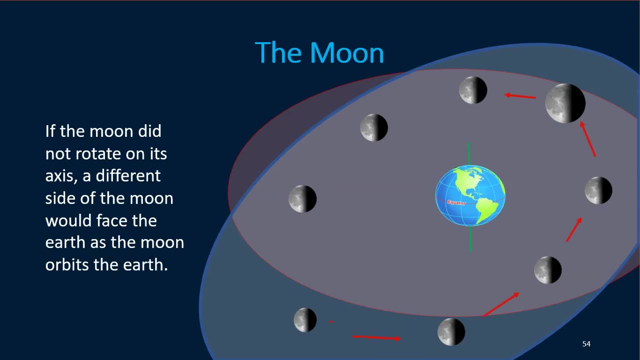 as it takes for it to complete one rotation on its axis, Because the Moon rotates on its axis at the same rate that it orbits the Earth. the same side of the Moon faces the Earth all the time. If the Moon did not rotate on its axis, a different side of the Moon would face the 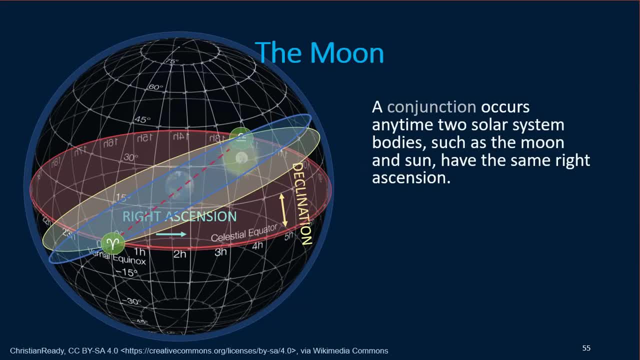 Earth. as the Moon orbits the Earth, A conjunction occurs any time two Solar System bodies such as the Moon and the Sun have the same right ascension If two bodies like the Sun and Moon have a similar appearance in size due to their 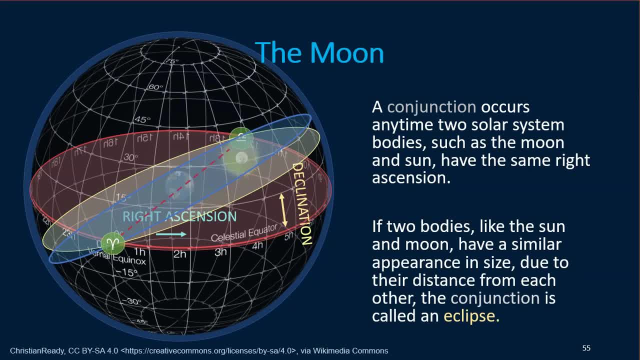 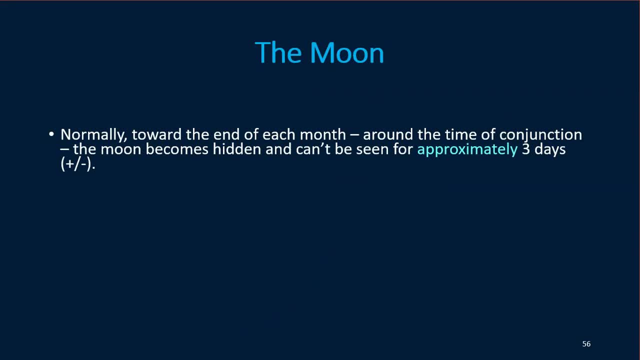 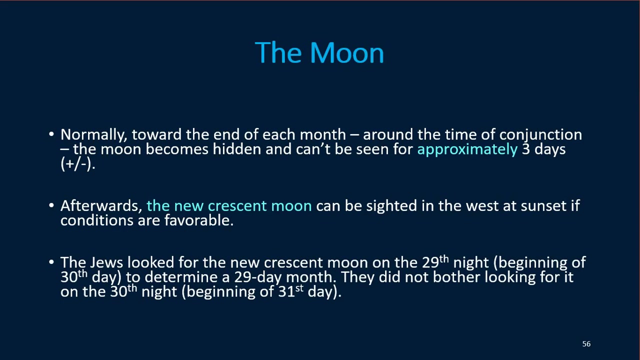 distance from each other. the conjunction is called an eclipse. Normally toward the end of each month, around the time of conjunction, the Moon becomes hidden. It can't be seen for approximately three days Afterwards. the New Crescent Moon can be sighted in the west at sunset if conditions are favorable. 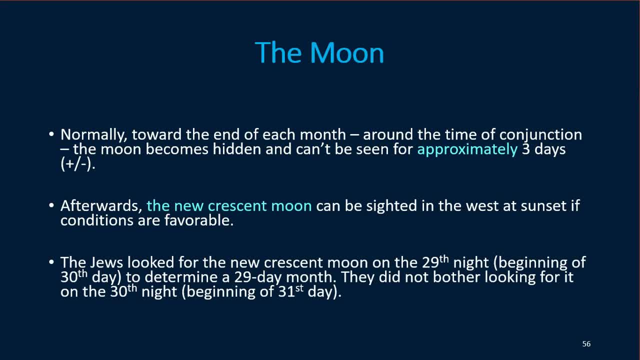 The Jews looked for the New Crescent Moon on the 29th night, beginning of the 30th day, to determine a 29-day month. They did not bother looking for it on the 30th night, which was the beginning of the. 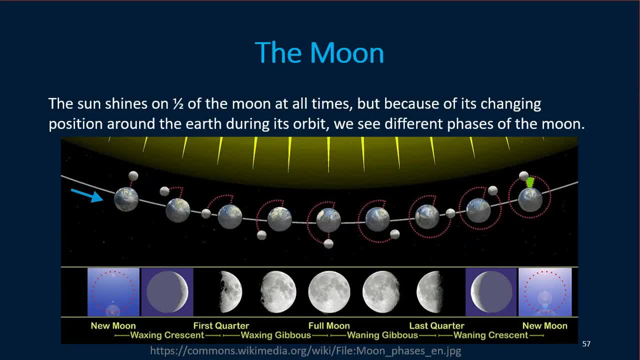 31st day. The Sun shines on half of the Moon at all times, but because of its changing position around the Earth during its orbit, we see different phases of the Moon. When the Moon is in this position, this is when we see darkness on this side of the Moon. 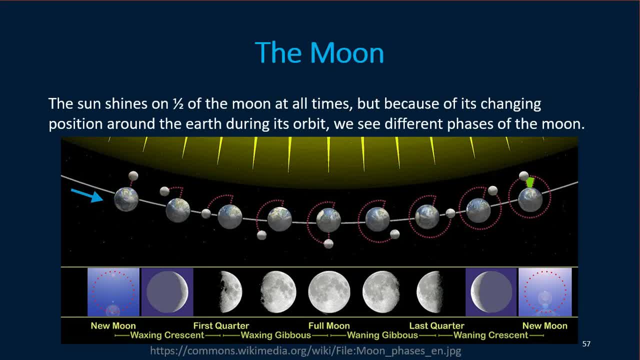 from the Earth. It's the New Moon, which is also known as conjunction. At this position, we're only seeing part of the light that's being shined on the Moon, and this is that New Crescent that we're beginning to see. 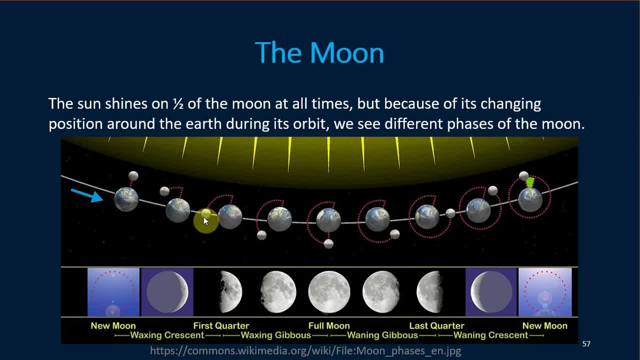 Next, when the Moon is in this position, we see the first quarter that looks somewhat like this. Then, when the Moon is at this position around the Earth, we see this waxing gibbous phase, And then, when the Moon is on the side of the Earth that's opposite that of the Sun, we 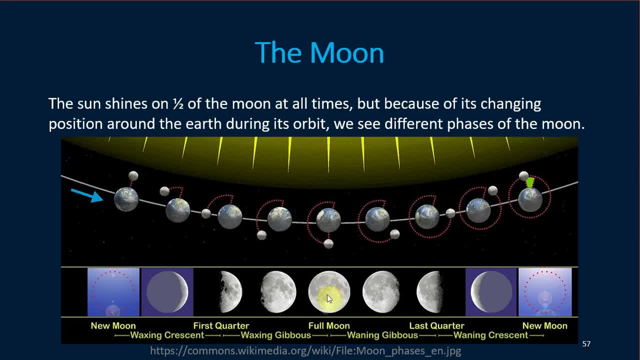 see a full Moon And then, when the Moon is in this position, we see a waning gibbous. And as the Moon continues to orbit the Earth in this position, we see the last quarter, and then, when it's about here, we see a waning Crescent. 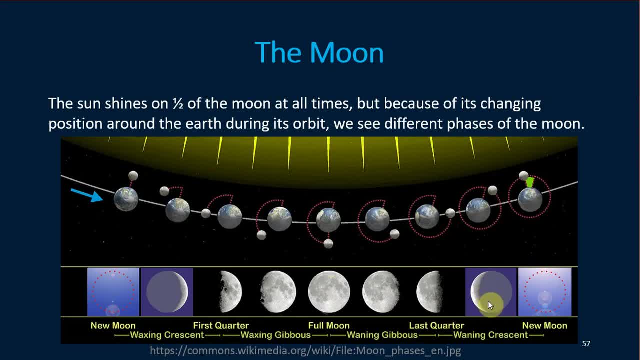 And then, finally, we have that conjunction again. Practically speaking, a Lunar month is either 29 or 30 days long, But a lunar month is either 29 or 30 days long, and then a lunar month is either 2 days long. 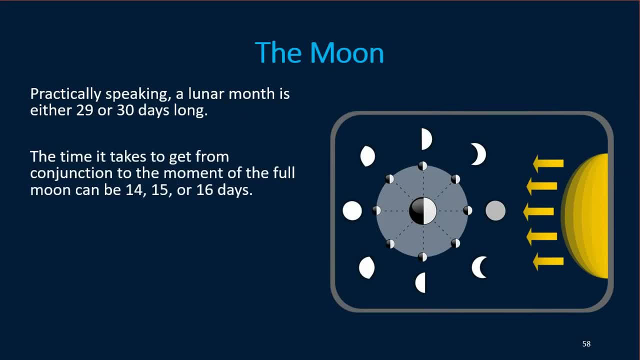 And then a lunar month is either 3 days long and then a lunar month is either 4 days long. the time it takes to get from conjunction to the moment of the full moon can be 14, 15 or 16 days. as a result of this variation, the feasts that take place on the 15th of the lunar month. 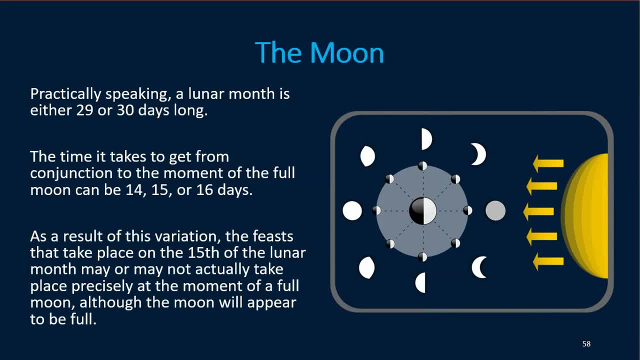 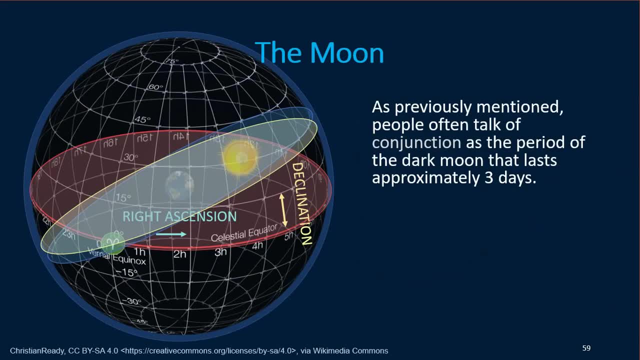 may or may not actually take place precisely at the moment of a full moon, although the moon will appear to be full. as previously mentioned, people often talk of conjunction as being the period of the dark moon that lasts approximately three days. this is okay, but actually conjunction is only a brief moment in time when the percent of illumination 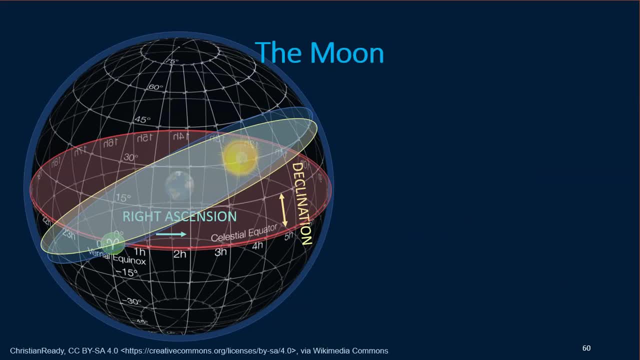 of the moon is at its lowest point. conjunction is also considered to be the brief point in time in which the waning crescent moon transitions to the waxing crescent moon. It takes place at the exact same time all over the world. The opposite of conjunction is full moon, which is when the percent of 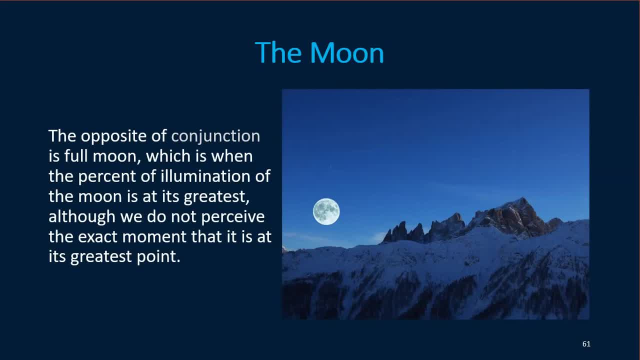 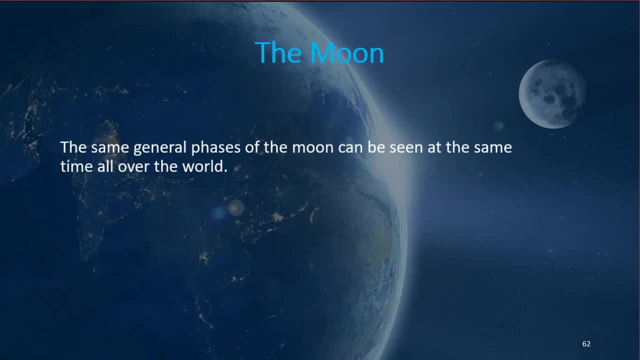 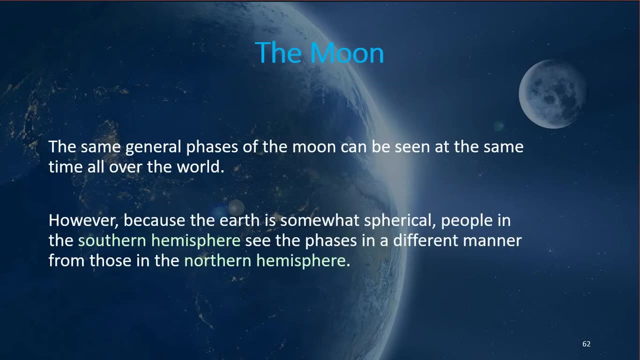 illumination of the moon is at its greatest, although we don't perceive the exact moment that it is at its greatest point. The same general phases of the moon can be seen at the same time all over the world. However, because the Earth is somewhat spherical, people 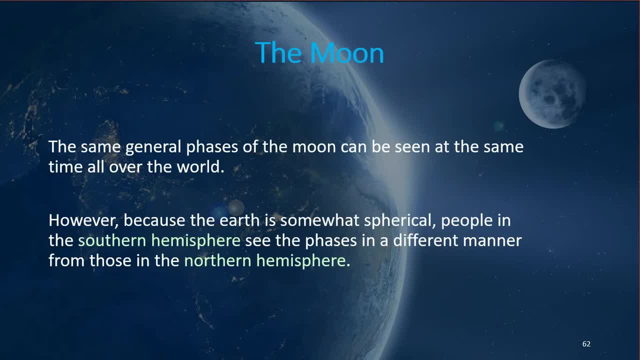 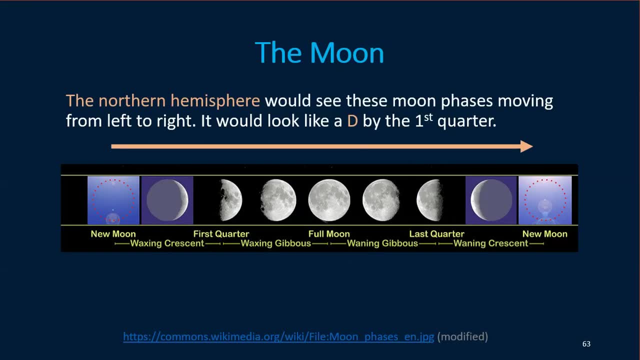 in the southern hemisphere see the phases in a different manner than those in the northern hemisphere. The northern hemisphere would see these moon phases moving from left to right- It would look like a D by the first quarter. However, the southern hemisphere would see them moving from right to left- It would look like a C. 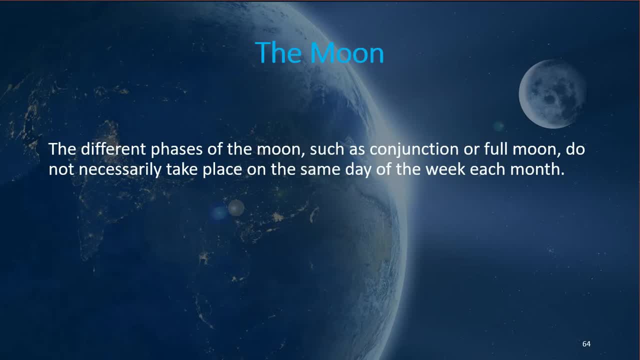 The different phases of the moon, such as conjunction or full moon, do not necessarily take place on the same day of the week each month. The only thing reliable is that the moon moves through each phase of its cycle over a 29 to 30 day period. 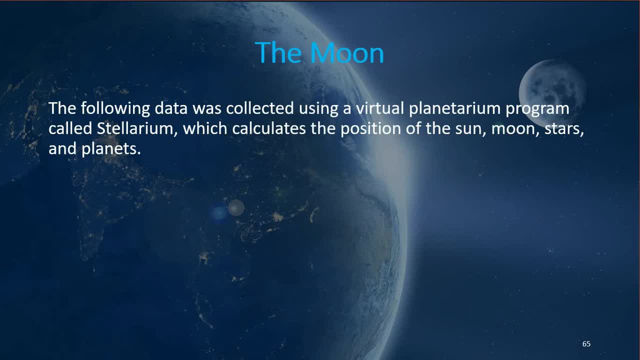 The following data was collected using a virtual planetarium program called Stellarium, which calculates the position of the sun, moon, stars and planets. Astronomers have been able and planets Based upon dates entered by the user. other data can be collected as. 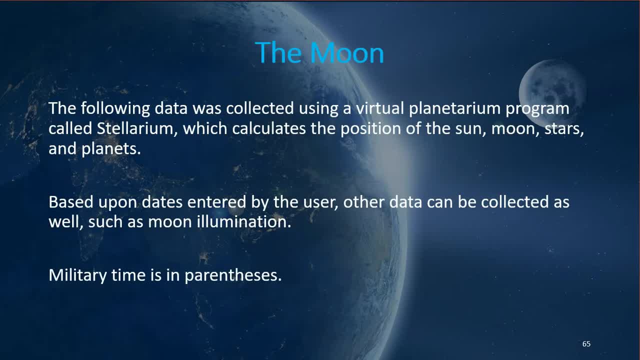 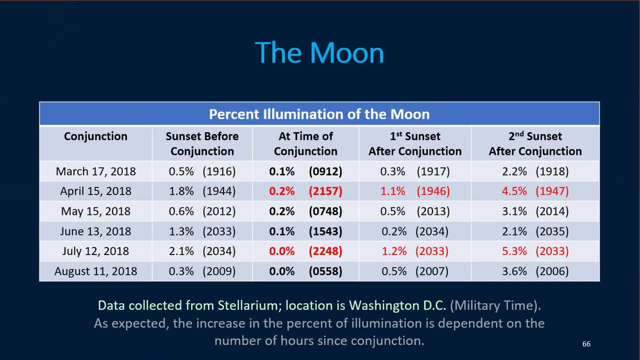 well, such as moon illumination. Military time is in parentheses. This chart shows the percent illumination of the moon on certain conjunction dates in 2018.. In the second column I have the percent illumination before conjunction and you'll notice, when you're comparing those to the time of conjunction, that 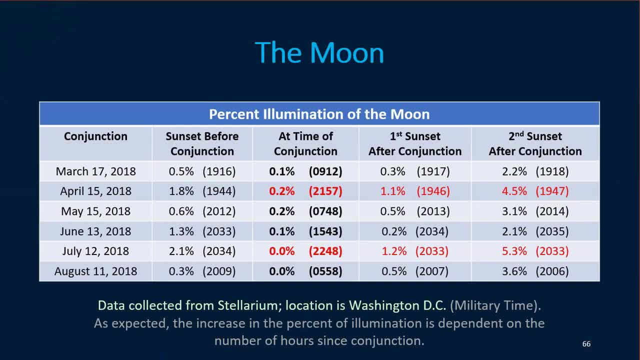 the illumination just before conjunction is a little bit higher than that at conjunction, and you'll notice that at the time of conjunction it's not always going to be 0.0.. It can be around that, such as 0.1 or 0.2.. I've also included 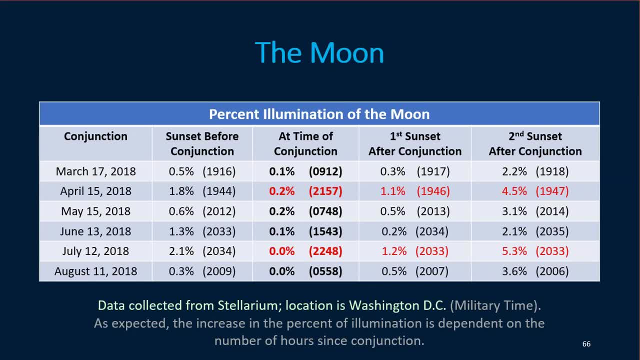 the illumination at the first sunset after conjunction- and this is going to vary quite a bit because of the amount of time that is between conjunction and sunset. You'll notice that the percent illumination is much higher at sunset when the conjunction is earlier in the morning. 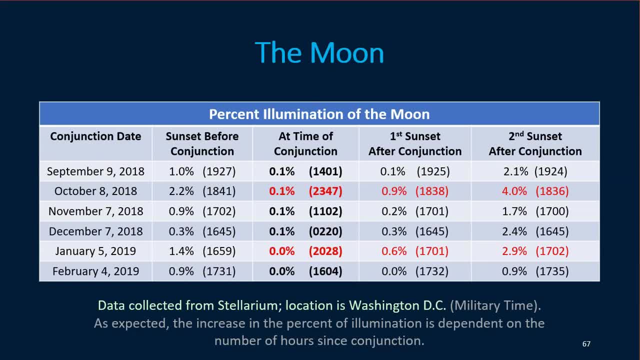 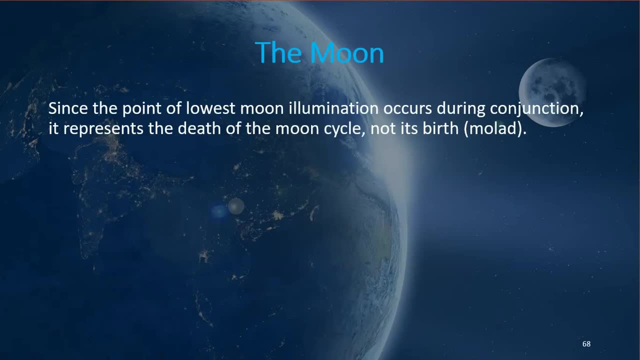 Here's the rest of the year. You may want to take a minute or so and stop the video and just kind of take a little time to look at these, in case you're interested. Since the point of lowest moon illumination occurs during conjunction, it represents the death of the moon. 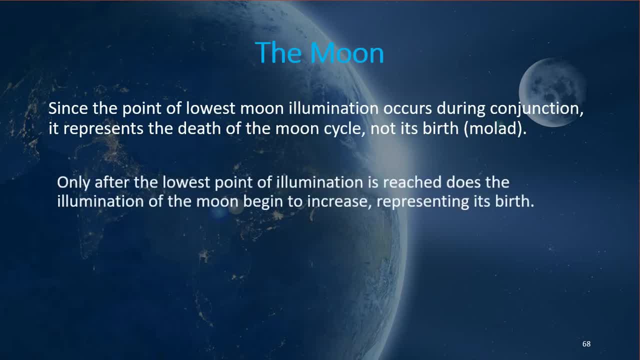 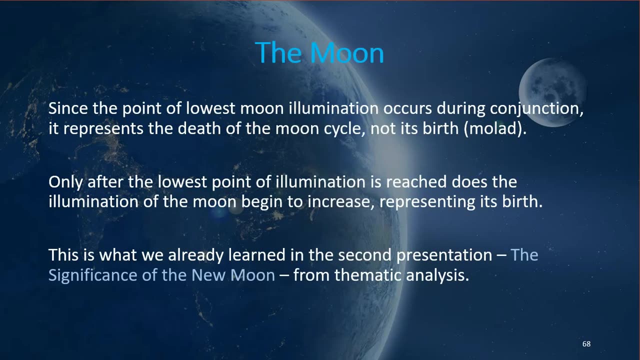 cycle, not its birth or milad. Only after the lowest point of illumination is reached does the illumination of the moon begin to increase, representing its birth. This is what we've already learned in the second presentation- The Significance of the New Moon- from thematic. 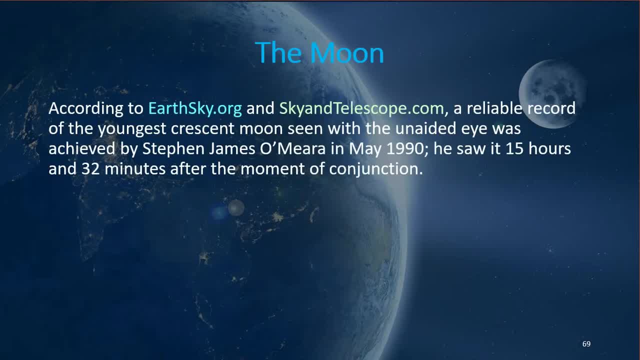 analysis At earthskyorg and skyandtelescopecom, a reliable record of the youngest crescent moon seen with the unaided eye was achieved by Stephen James O'Meara in May 1990.. He saw it 15 hours and 32 minutes. 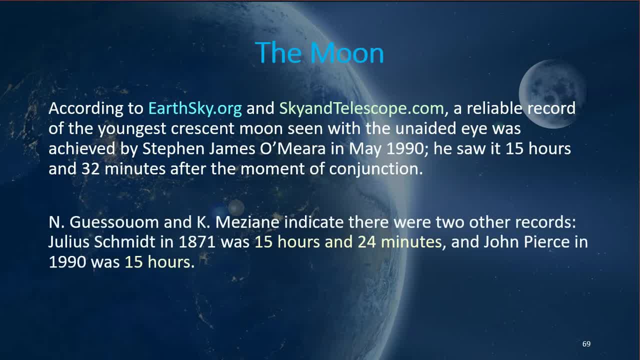 after the moment of conjunction: N Gesuom and K Mezian indicate there were two other records: Julius Smit in 1871 was 15 hours and 24 minutes And John Pearce in 1990 was 15 hours. 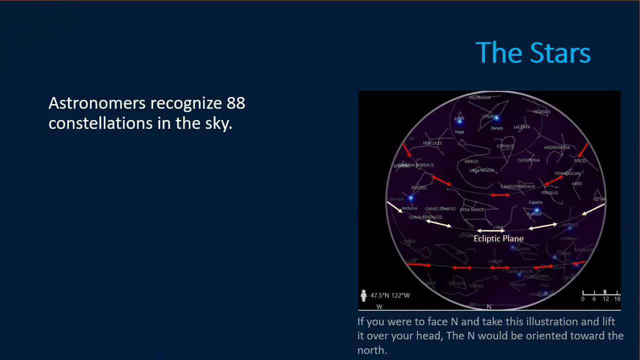 Now we'll talk about the stars. Astronomers recognized 88 constellations in the sky. Some constellations are specific for either the northern or the southern hemisphere. These constellations are circumpolar or positioned around one of the Earth's poles. 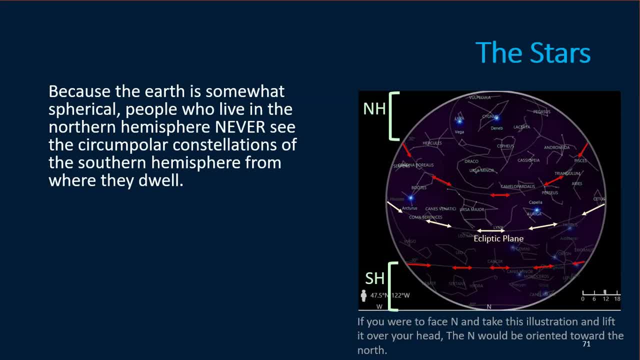 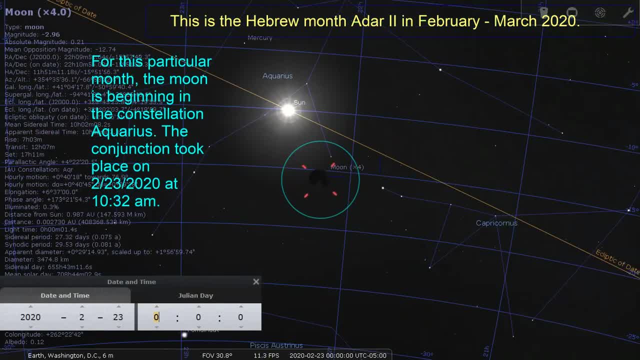 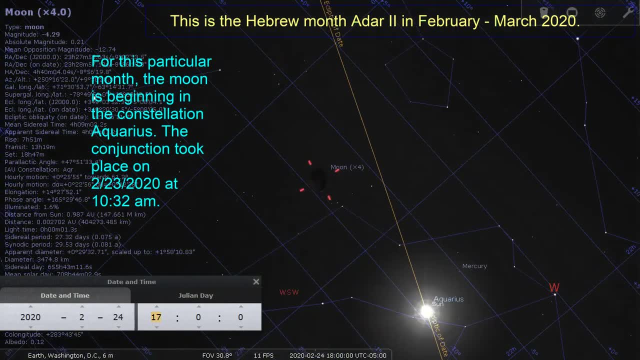 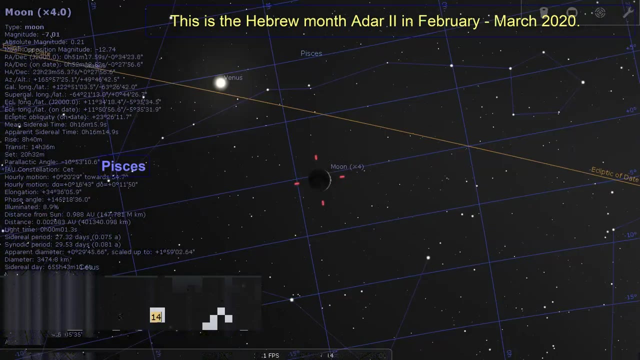 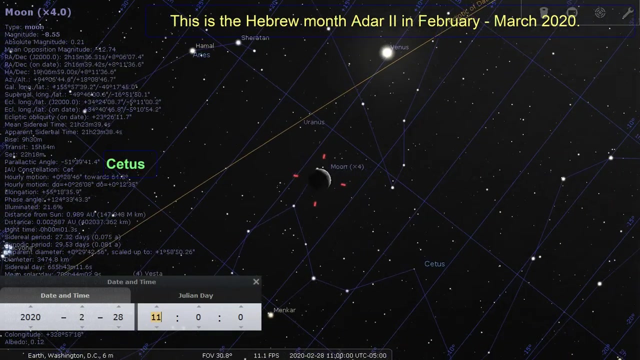 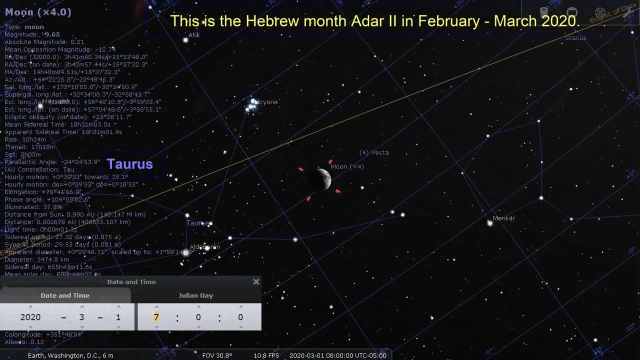 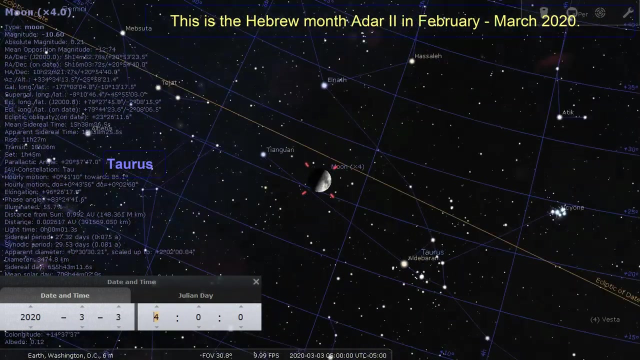 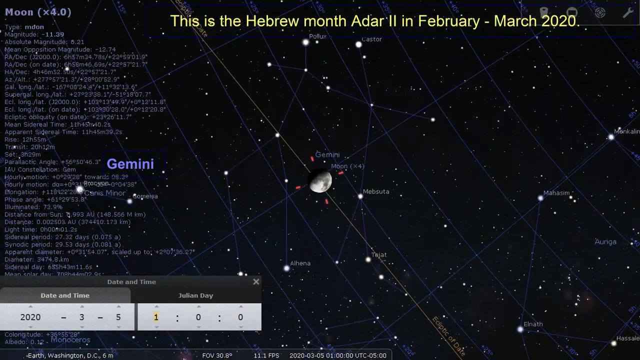 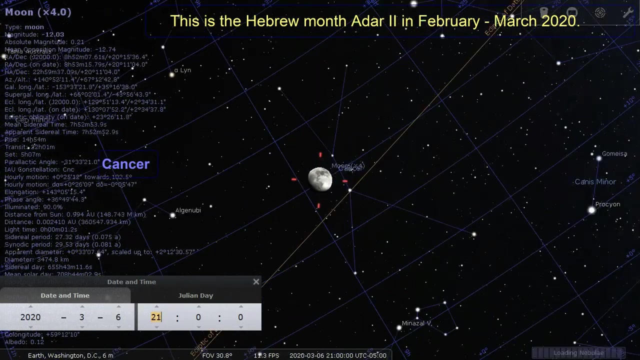 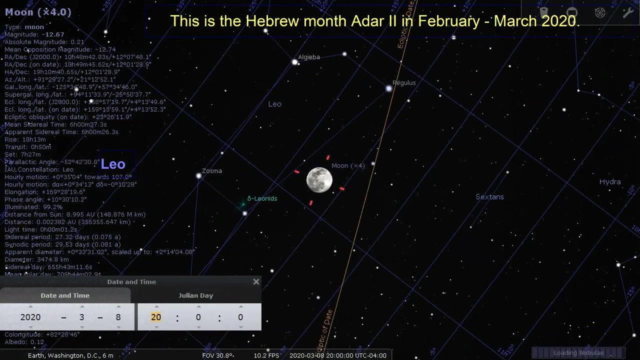 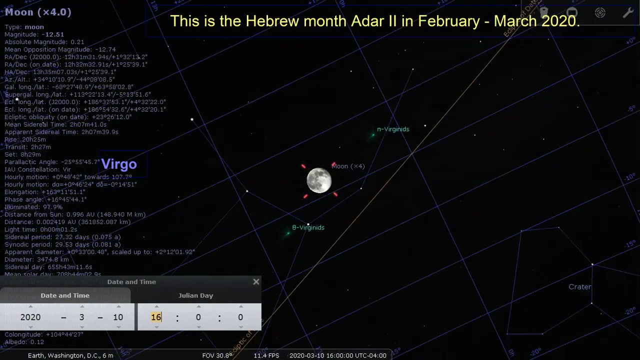 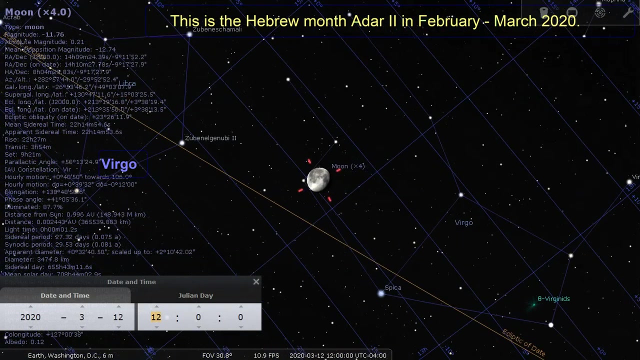 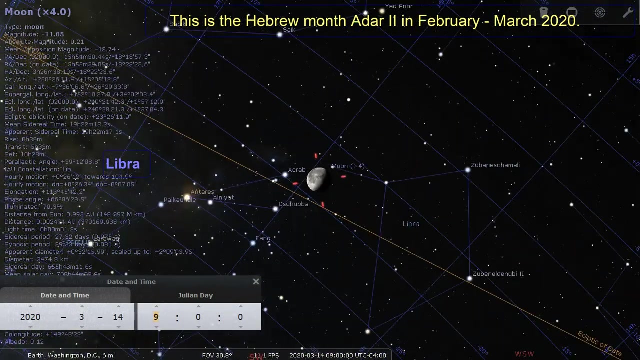 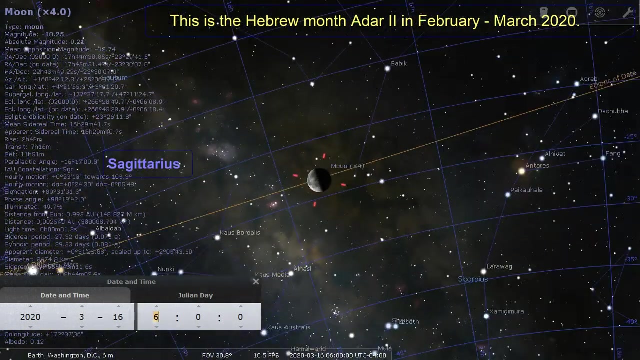 People who live in the northern hemisphere are more likely to see the stars. People who live in the northern hemisphere are more likely to see the stars. Thank you for watching. Subtitles by the Amaraorg community. wwwamaraorg. Subtitles by the Amaraorg community. Now we're about to look at the Sun as it appears to move through the zodiac in a year for a regular year, followed by a leap year. Now we're about to look at the Sun as it appears to move through the zodiac in a year for a regular year, followed by a leap year. Now we're about to look at the Sun as it appears to move through the zodiac in a year for a regular year, followed by a leap year. Now we're about to look at the Sun as it appears to move through the zodiac in a year for a regular year, followed by a leap year.